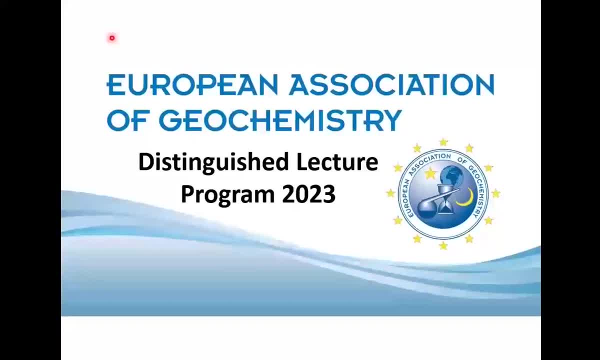 Yeah, thank you very much. First, I would like to thank the European Association of Geochemistry for inviting me to this lecture tour and thank you very much for hosting me here and giving me the opportunity to talk a little bit about my research, my educational background. 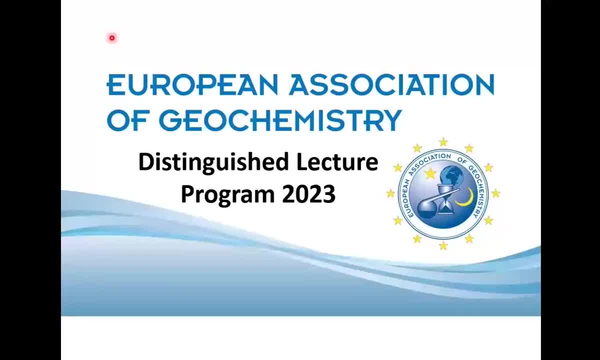 So I've done my bachelor's and master's in Germany at the Katharine Osietzky Universität in Oldenburg, then went on to do a PhD at the University of Utrecht in the Netherlands, moved on to do a two-year postdoc at the LMTG in Toulouse and from there moved on to the University of Bristol, did a postdoc and then had an assistant professor position and then, in 2017, moved to the University of Utrecht. 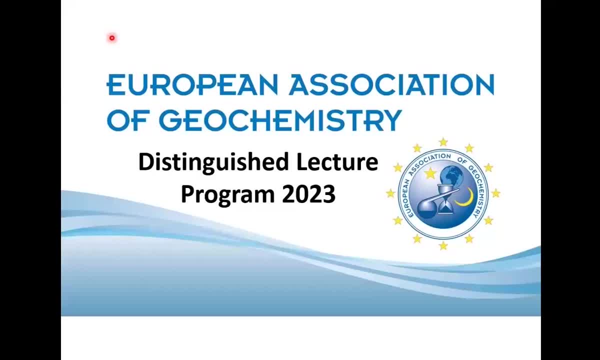 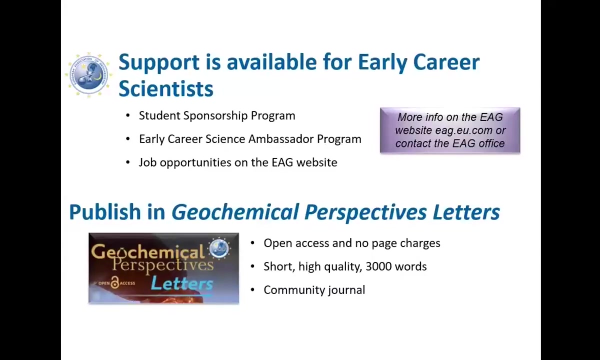 So, as already mentioned, my research focus is largely on carbon cycle and climate effects, but before I go into detail about this, the AG has asked me to provide some additional information. There's a lot of support available for early career scientists from the EIG, namely sponsorship programs, a really good early career science ambassador program. 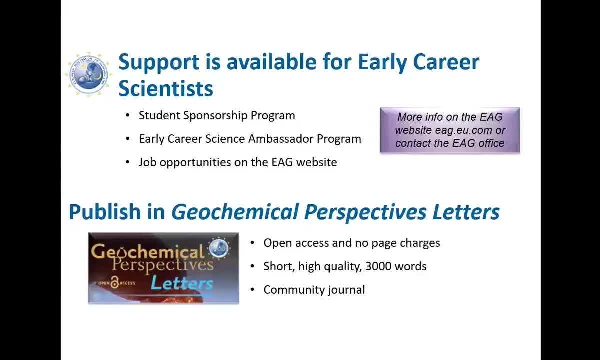 There's a really nice job portal on the EIG website. You can find a lot of information about all of this here on the website or by contacting the office, So if you're motivated to do that, There's also a community journal: Geochemical Perspectives Letters. 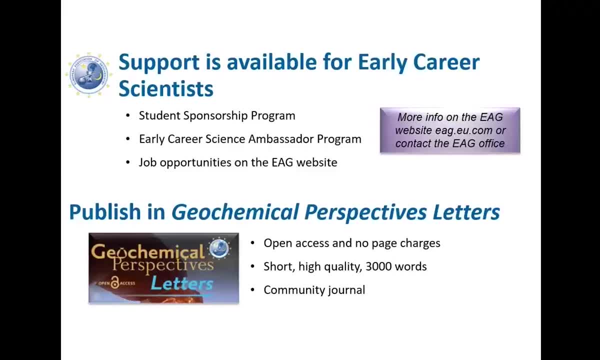 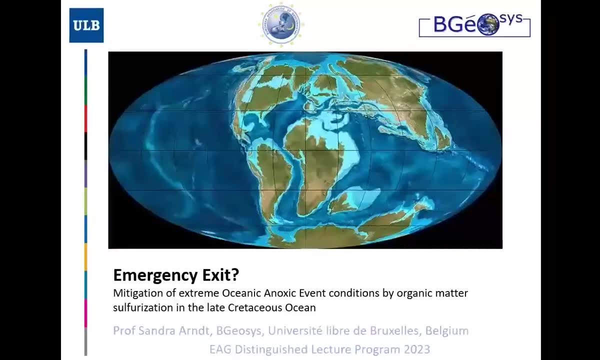 It's open access and has no page charges, so it's going to be for free, has a short article, a few words and generally of high quality. So take that into consideration. And now to the carbon cycle and climate context. So in the first lecture I want to talk a little bit about past climates and past climate events, namely oceanic and noxic events. 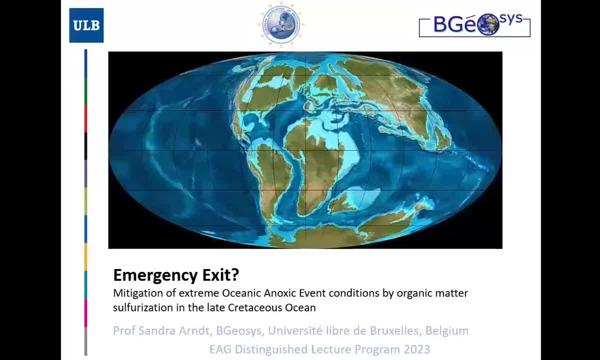 That's early Cretaceous, when the Earth looked a little bit more like this, And specifically, we're focusing on the conditions that led to the start of the termination of these carbon cycle climate perturbations in the Cretaceous and how we, through a very 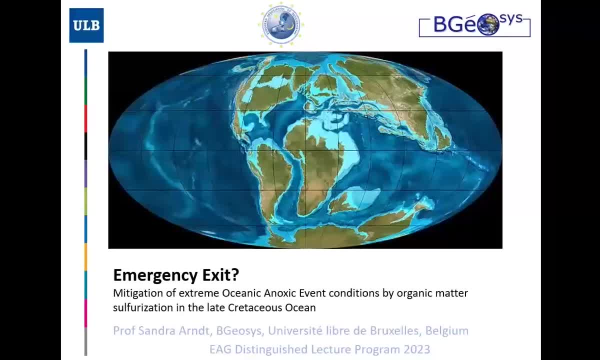 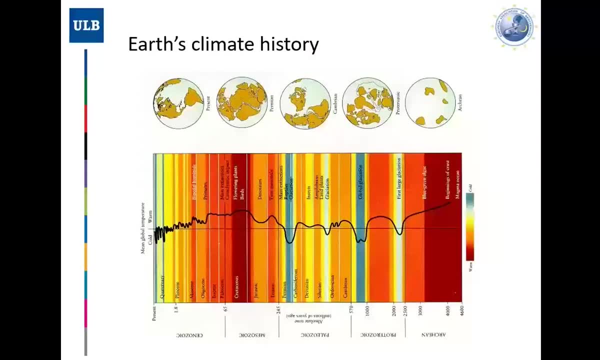 multi-step integrated model data approach, got to learn a little bit more about how the Earth's system responded to this condition. So when we look at Earth's climate history, we can see this. It's kind of we can see this sequence of warm and cold periods that just follow each other, though sometimes a little bit more extreme than others, and a big interest in all of this is like: how did the climate system respond to these perturbations? 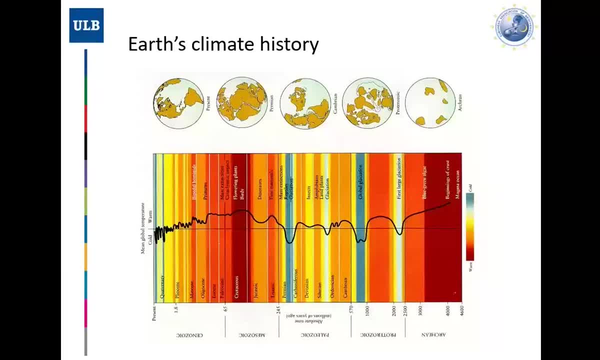 What were the triggers of these perturbations and the timescales of these perturbations? And this is particularly relevant nowadays because we are we're facing like a very rapid perturbation of the climate system caused by anthropogenic activity, and looking at these past periods really can help us understand how the Earth's system can react, how the carbon cycle can react and did react in the past to these often much more extreme, even though on slower timescales, carbon cycle perturbations, climate. how did the Earth's system recover from these extreme events? 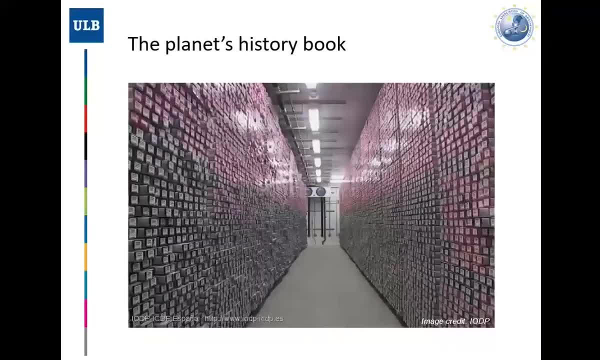 How can we find this out? Well, luckily, the Earth's system is writing its own history book. Here you can see these are sediment cores that have been collected and drilled all over the world. They're stored in a core repository. There are multiple around the world. 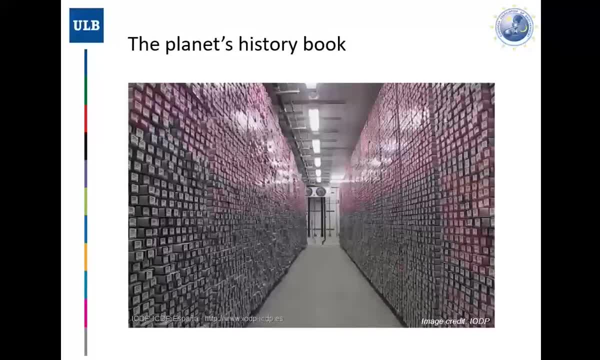 So these ones specifically, they come from the ocean drilling program, So it's like a deep sea drilling program that can recover sediment cores of considerable length up to kilometers Down in really deep water depths, so out in the deep ocean. That's a history book of the Earth's, so it's been recorded in the sediments and then, once the sediments get uplifted, obviously in the rock record as well. 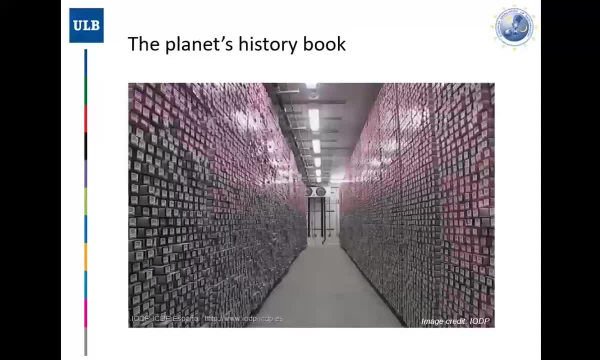 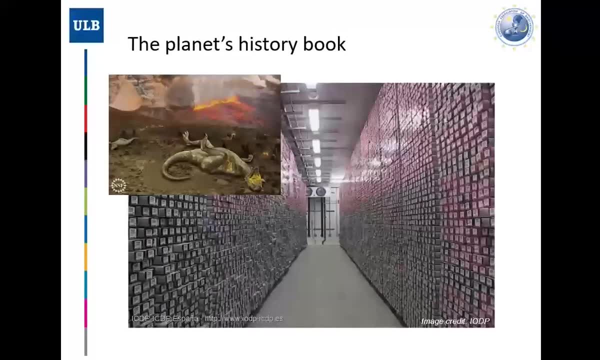 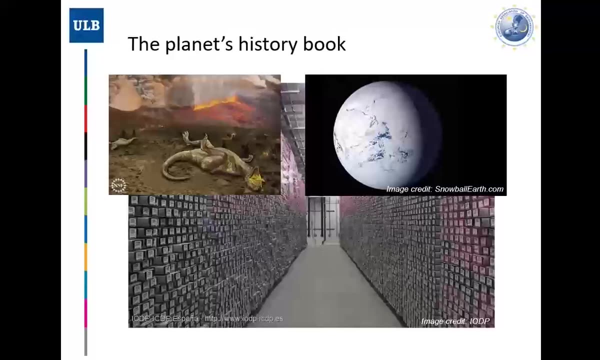 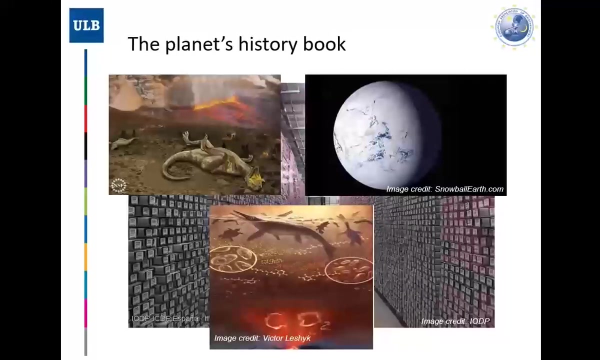 But I will focus most on the zoic climate, which is recorded in the sediments and this history book records, like the stories of extreme mass extinctions, extreme events and extreme classiations in Earth's history. This is obviously not recorded in the fungal and zoic sedentary rockers but in the rock record. this is the neocontrolozoic snowballers and really really different ocean environments from where we are now, like oceans that were highly sulfidic and hoxic. 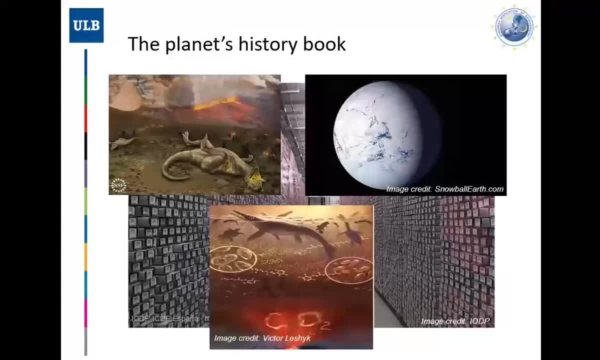 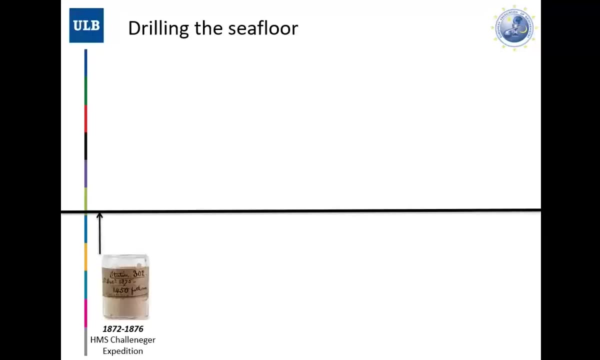 So you would say, well, that's great. So the Earth's system is recording its own history, so we should know quite a lot about it, Since we have access to rocks and sediments on Earth. the thing is like the sea floor, for a really really long time, was considered as a desert, a pretty sterile environment, not much going on, pretty boring, so nobody was really interested. 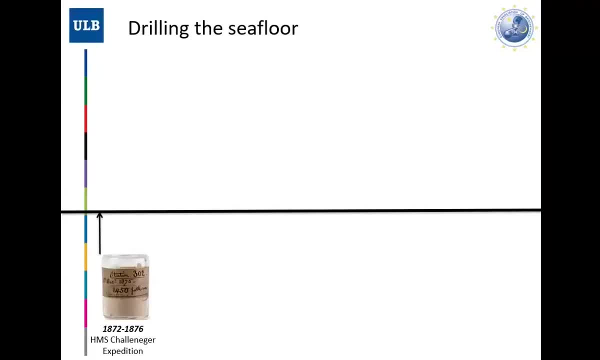 And then interest kind of started only in the middle of the 19th century with a big hypothesis that we formulated about past ice ages And we also did a lot of research into the past climate, possibilities of past climate change, the theory of evolution and things like that. 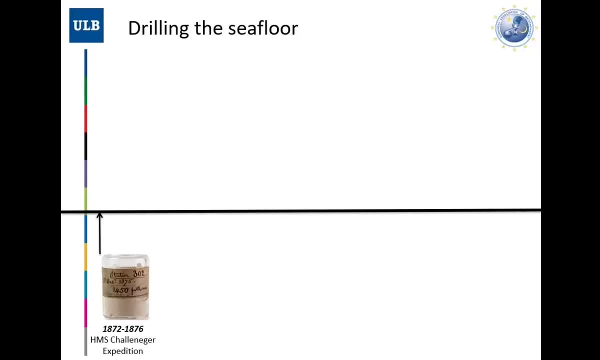 And the first marine expedition was a MHS Challenger expedition we had towards the end of the 19th century and they recovered a few hundred trash samples or just sediment samples, but not much done with this. So even at the end of the Second World War, in 1942,. 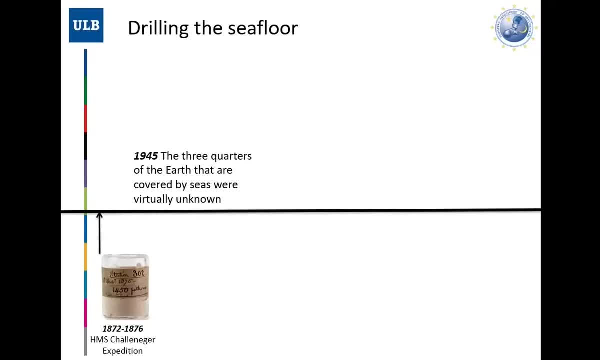 The three quarters of the Earth's surface that are covered by oceans, that are covered by water, were virtually unknown. We didn't really know what was there. we didn't really know all of the kind of Earth's secrets and Earth's history that was recorded in the studies. 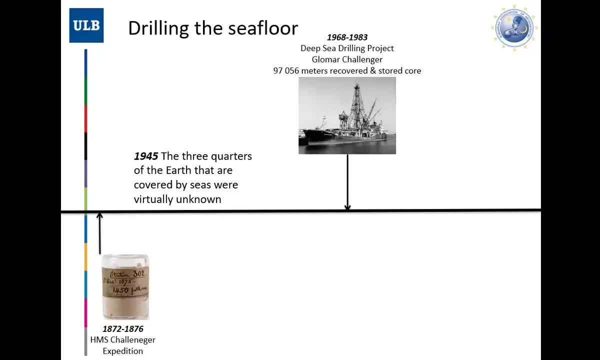 And that drastically changed with the beginning of the Deep Sea Trilogy Programme in the 60s. That's also where the Ice Age theory was then confirmed and developed. They recovered almost 100,000 metres of sediment cores and stored these cores, so providing a lot of information about past climates, past environments and climate history. 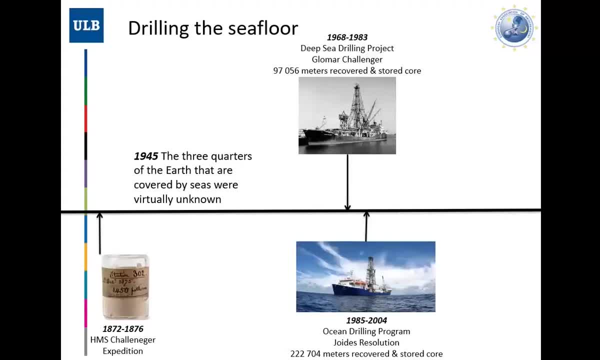 This was followed by the Ocean Trilling Programme running from the 80s to 2004.. It's a joint resolution. We're covering a further 200 or more. We're covering 200,000 metres of sediment records, Followed by the Integrated Ocean Trilling Programme, which ran until 2013.. 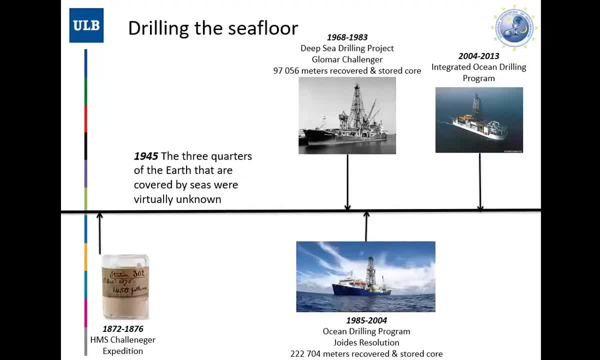 We're covering even more deep-sea sediments. By then, we already developed quite a good understanding of a lot of the past events, especially through the analysis of these sediment cores And then, since 2013,, the International Ocean Discovery Programme. 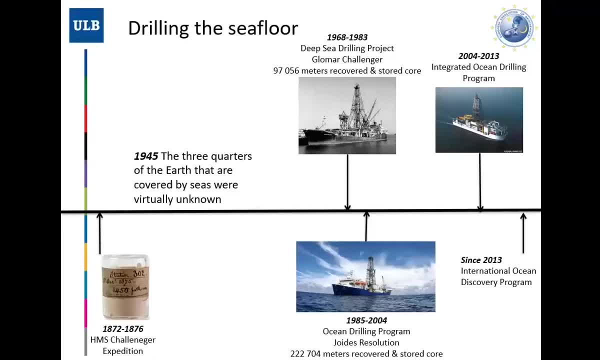 So the point is that these deep-sea drilling activities really provided us with a lot of information about past climates And, as Charles Hutton said, the present is the key to the past. We can also see that this past information about these past climates is also the key to the future, to understand how the carbon cycle can respond to these extreme conditions. 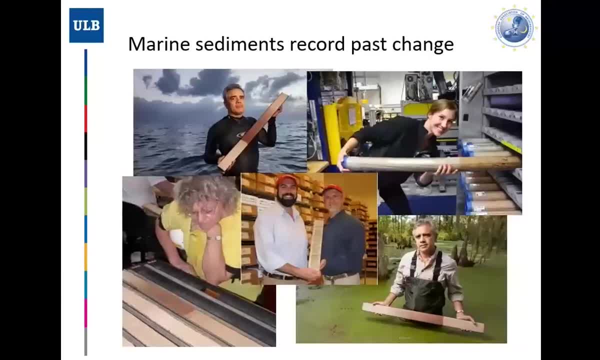 So sometimes you can already tell that there's a lot going on. There's a lot going on. There's a lot going on, But you can already clearly see. So you might wonder why all these people are taking photos with sediment cores. 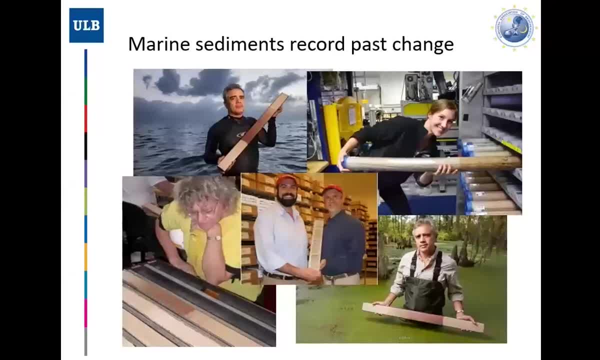 But you can see, here it's a very clear difference. This is Paleocene-Eocene Thermal Maximum And here you can see the PTM, which is basically a marine or ocean acidification event. So you can see like it disappears. 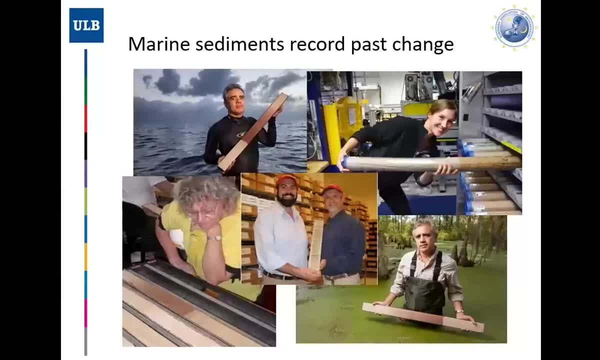 It's calcareous sediments, limestone sediments. It's completely limestone-free in the world And this is reported in different locations around the globe as well. So sometimes these changes are very obvious in the sedimentary record. You can visually see that. 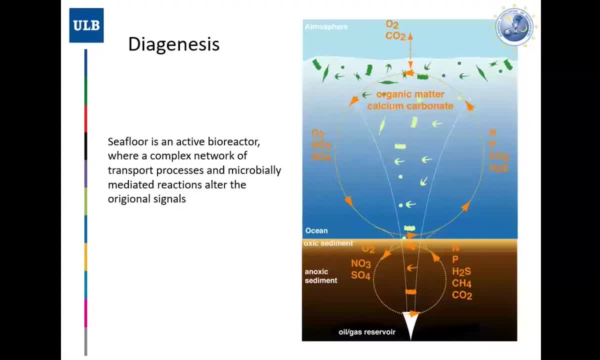 But very often that's not necessarily the case. This history book is a little bit difficult to read, As you can see, if you have material that settles down into the sediment. it's not just sitting into the sediment And, contrary to the past view that the seafloor is a sterile desert where nothing happens, there's actually a biogeochemical reactor. 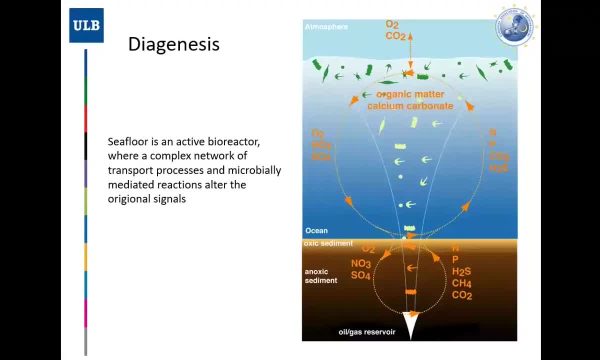 There are early diagenetic processes that kind of degrade organic material, consume terminal electronic samples, release metabolites, precipitate autogenic minerals. They kind of alter the sedimentary record. So this primary signal we are reporting is altered And that makes it sometimes very, very difficult. 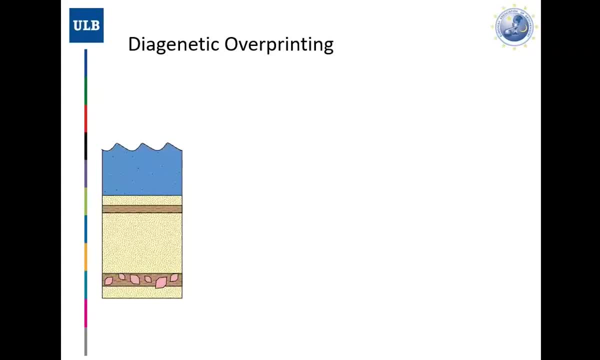 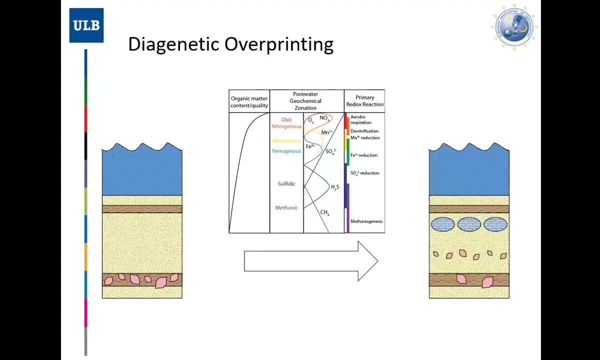 So you can see. it's something like that. So I have a rift here that's deposited And then, with the action of diagenetic processes in this upper sediment area or deeper even later, you will have like a consumption of this signal here. 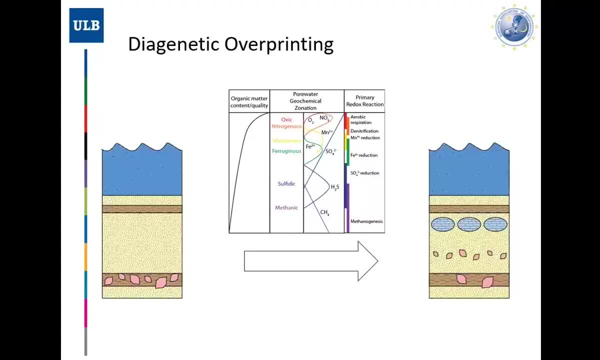 For instance, I put some organic material in each layer With some mineral inside, And then the re-precipitation of these minerals that dissolve down here, Or even new precipitation of autogenic minerals in a completely different location. So that makes it really really difficult at times. 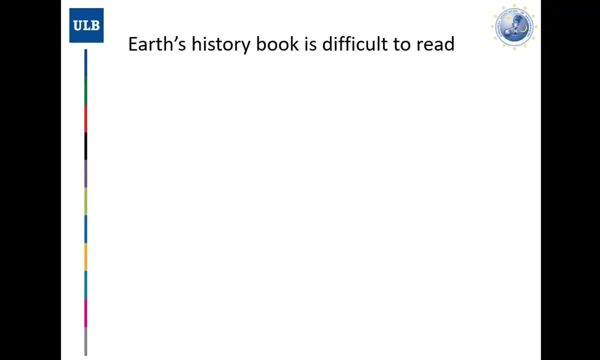 So the Earth's history book is pretty difficult to read, It's not only difficult to reach, So you have to have a research vessel that can drill deep into the sediment, Because the deeper we drill into the sediment, the further we go. 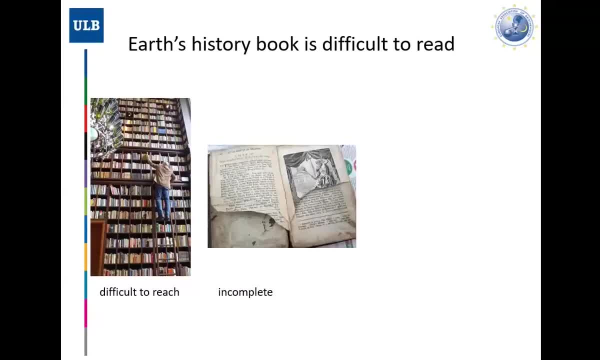 It's often incomplete, like the rock record as well. There are things missing. Maybe there was no sedimentation, Maybe something was eroded, Maybe something just was consumed and disappeared over these times, And the thing that makes it really really difficult is that things have been added later. 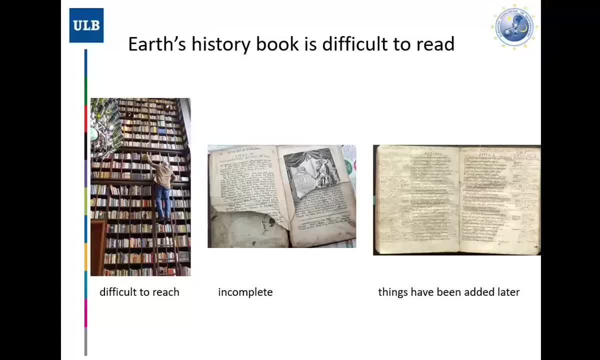 So there have been processes in the sediment that have acted over these long times, So they have overwritten or written new things into this history book. So that makes it very, very difficult to go back and say like, well, this is how the environment looked, let's say, 100 million years ago. 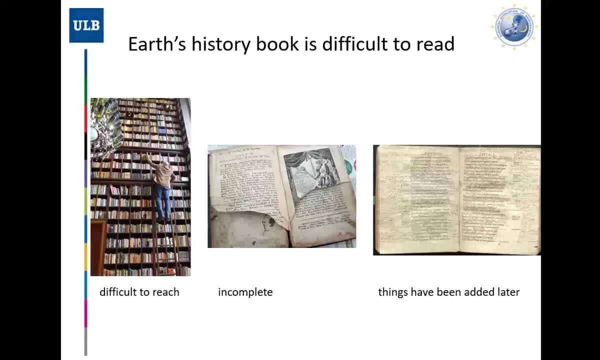 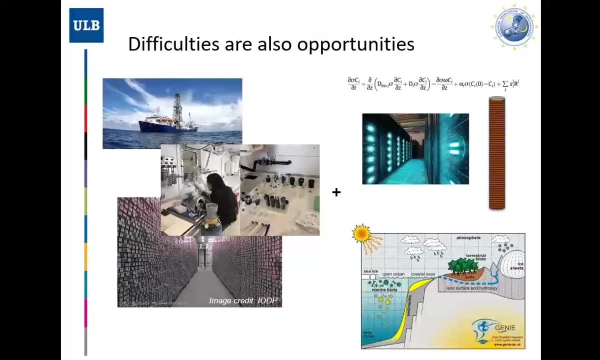 And this is the original signal. This is what was deposited at this time and at this place. So pretty difficult. But difficult is not necessary. Difficult is not necessarily bad Difficulties. you should see difficulties always as opportunities. So there are things that make it very difficult. 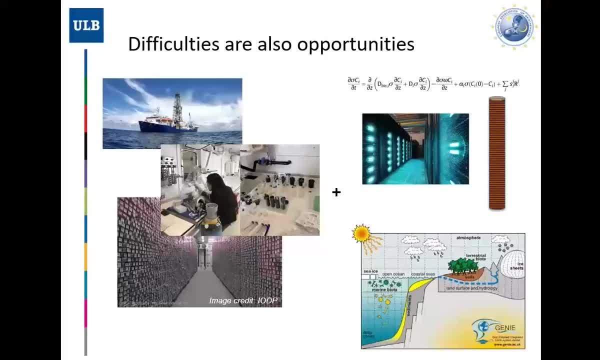 But these things that make it difficult might also contain very, very useful information, And today, in this talk, I will show you how we use that in a combination with like observations. So from this drilling, from these sediment records and specifically through extracting pool waters from these sediments, 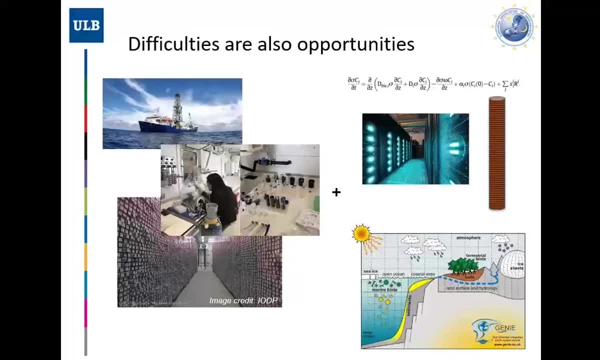 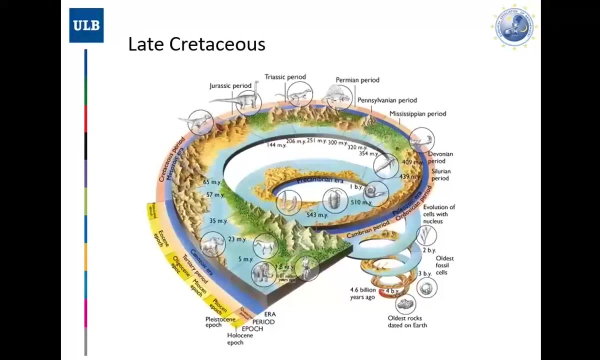 Analyzing the solid-phase sediment and combine that with numerical modeling to really unveil some of the secrets that were recorded in these sediment cores. And I want to take you back to the late Cretaceous, So that's about 100 million years ago. 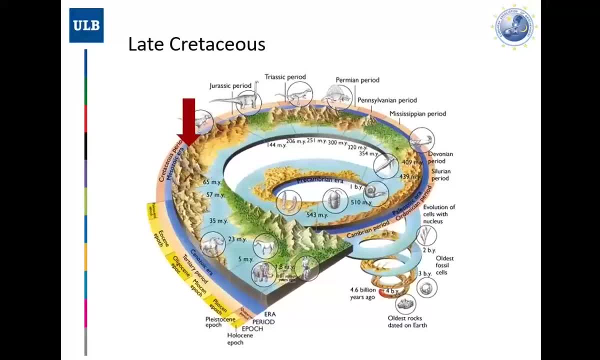 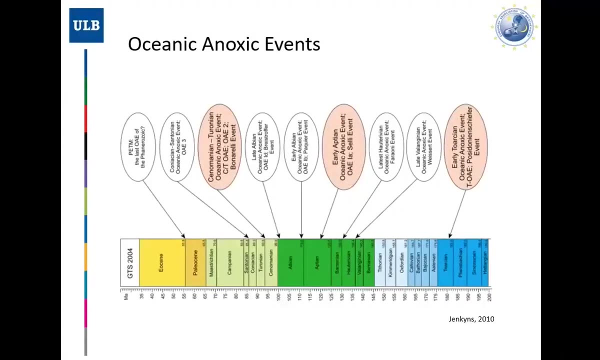 That's about the end of the era of the dinosaurs, So there's a big impact. when the dinosaurs disappeared, It's around this time, And the Cretaceous is a specifically interesting period in the geological past Because it's really spiked by a lot of these oceanic unobstructed events- OAEs, they call them. 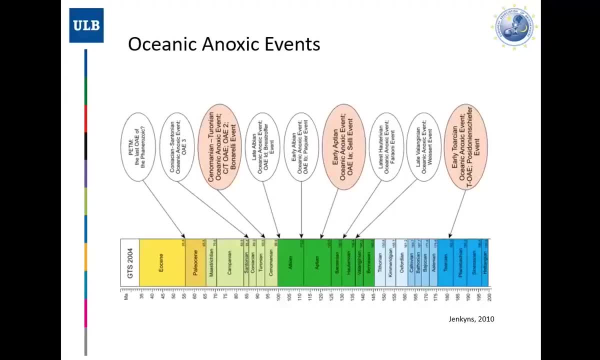 So they were discovered a long time ago, But formerly, like Flannan Jenkins, they coined the term. They occur in different at different times of Earth's history as well, So you can see here, for instance, PGM sometimes. 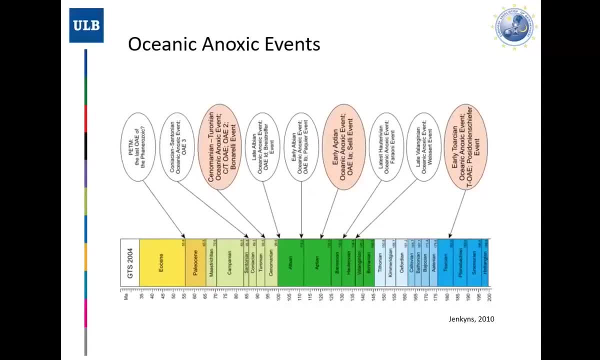 Ophagalus OAE as well. There have been other events, The Ibonian as well, The Calabasa event, for instance, But the Cretaceous is specifically prominent because it has a series of events And at least these events here highlighted in orange are confirmed to be global events. 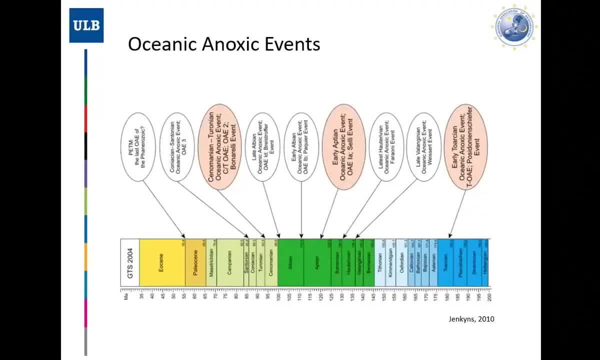 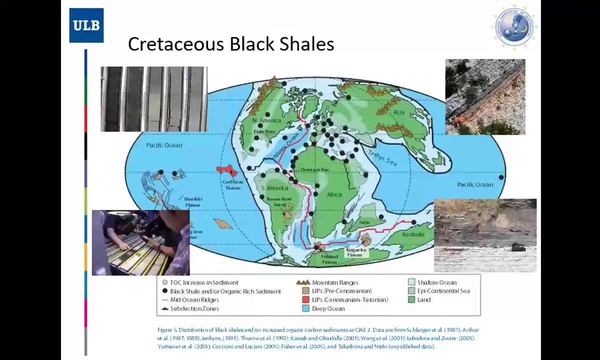 So global events, global extreme carbon cycle, climate perturbation that affected the whole Earth and all geochemical records, And first they were kind of identified by black shales, So Cretaceous black shale, So you can see that here. 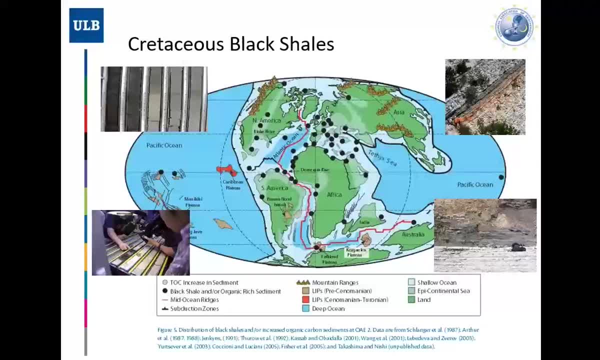 It's a little bit like with the PGM. It's a specific layer you find every time you drill somewhere and you find Cretaceous sediments. It's organic, A matter-rich layer. They can have organic matter a content of 1 to 30 weight percent. 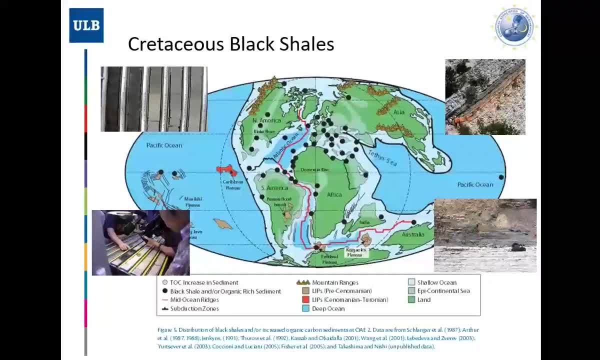 So quite rich, Especially here in the deep chilling sites in the Atlantic, but also in the Pacific, on the past Submarine volcanic plateaus, And then outcrops and lands, especially specifically in the Apennine area of Italy, And here you can also see it's normally a lot of limestone as well. 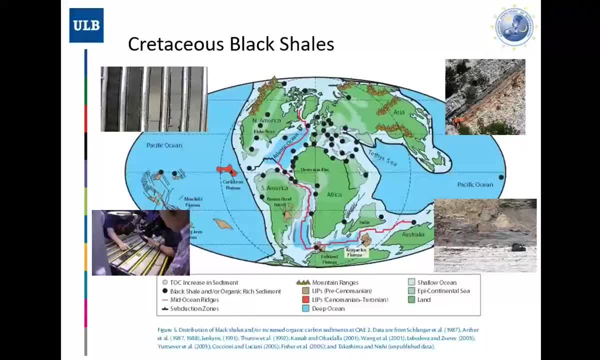 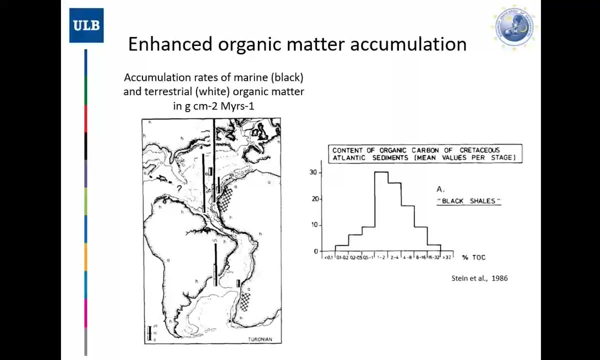 And here you can really nicely see this black shale layer. So global occurrence was specifically a higher evidence of frequency of black shale occurrences in the Atlantic and sometimes the Pacific. What we see is also this type of enhanced raise of marine as well as terrestrial organic 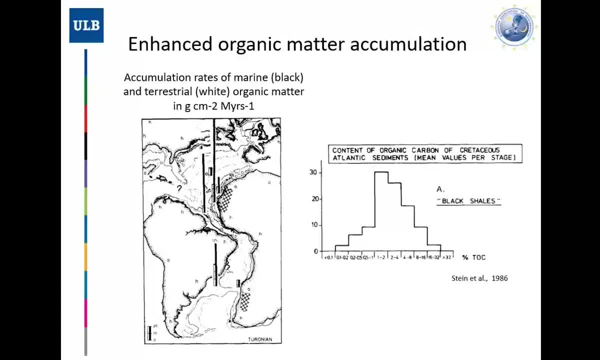 matter accumulation in these areas. Here are estimates And you can see here the distribution of organic carbon content in black shales. This is a huge variability, which are really a tendency to enrich organic carbon content, But sometimes that's difficult. So just identifying Cretaceous black shales on the basis of organic carbon content is a little bit tricky. 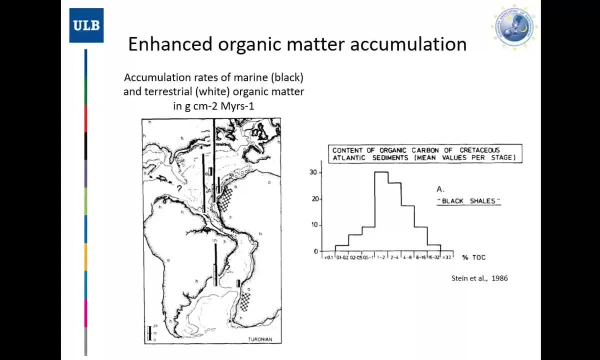 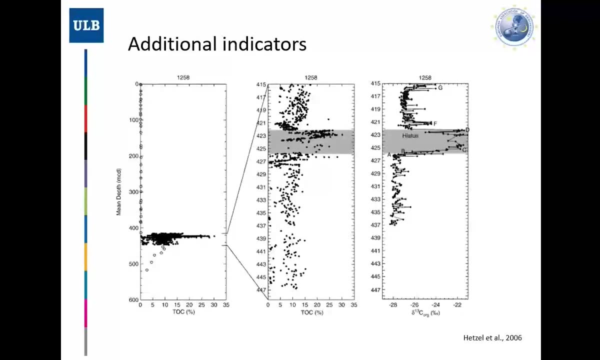 because it can be diluted. So you can still record an OAE event without having a black shale, because the organic carbon deposition can be diluted by high sedimentation rate or the organic carbon maybe was just consumed in the period that passed. There are other indicators except for this high organic carbon content. 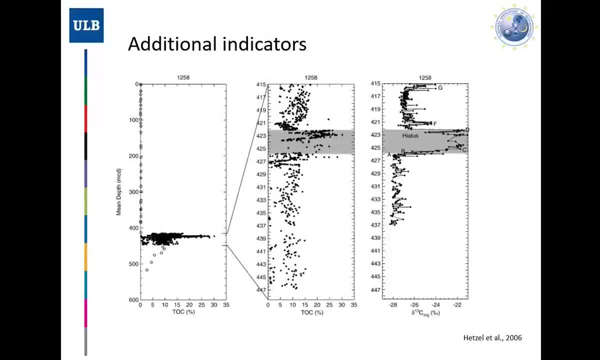 So here this is data from Demerara rice, So I will talk a little bit about Demerara rice later. It's OGP 207.. It shows Cretaceous black shales in this area. So here you see the sediment depth. 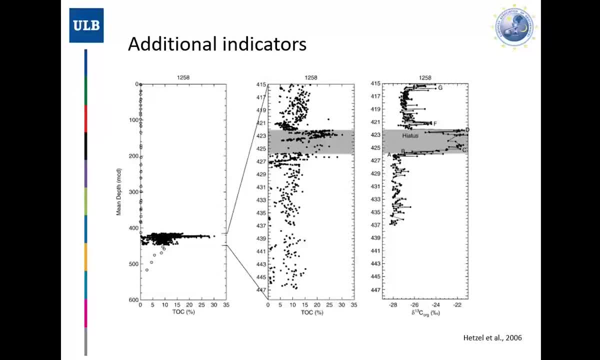 Yeah, 450.. Yeah, So you can see here the sediment depth. There's this Cretaceous organic enriched layers with organic carbon content up to 30%, And what you also see like here's the high resolution in this layer. It's like there's a positive excursion. so much like the delta C13 values in the organic 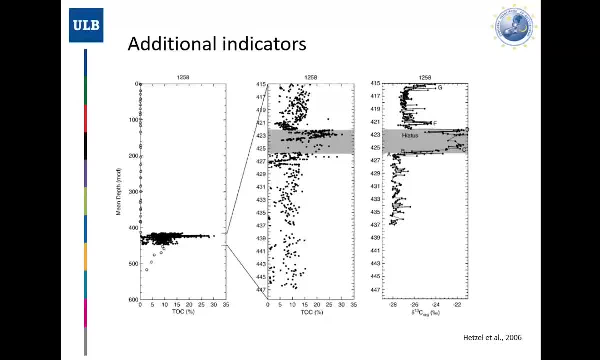 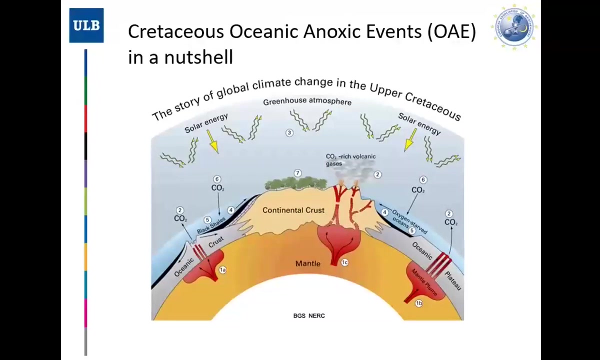 matter And that's very typical. So typical marine is 25, 125.. What you see here is like a very high resolution. it's like an indication for a major burial of organic carbon, thereby making the remaining pool much more heavier in the water column. So what happens during these anoxic events? We have a 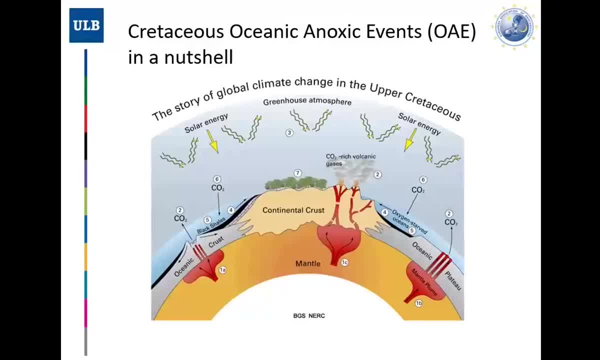 pretty good understanding nowadays when we think how these events unfolded and how they finished and ended. So this is a mutatious, anoxic event in the nutshell. So what we think was the trigger is it's probably an increased volcanic activity, mantle activity- that leads to an increased 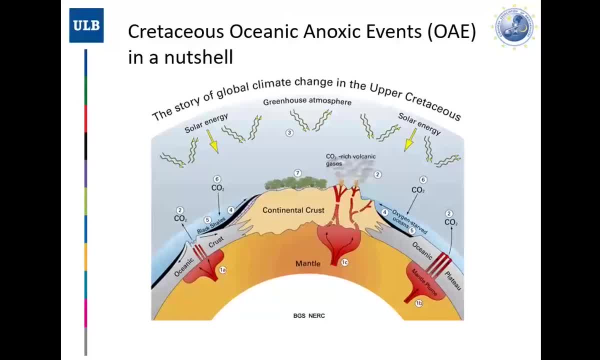 volcanic activity, enriching the atmosphere and CO2 and creating a quite extreme greenhouse gas, a greenhouse climate, with greenhouse gas or CO2 concentrations in the atmosphere about 3 to 4 minutes. So that's what we think. So what we're trying to do is to try to find out how these events 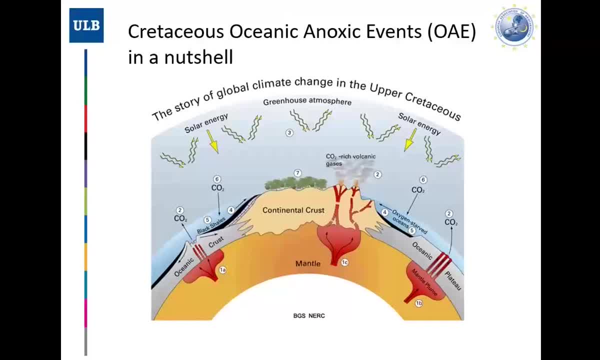 unfold. So we have an environment where you have dense weathering rates. you have a dense hydrological cycle bringing nutrients out into the ocean. This sparked, like, increased primary productivity in the ocean. you have more material that sinks in the ocean than gets degraded by bacteria in the ocean. These bacteria use oxygen in the ocean. 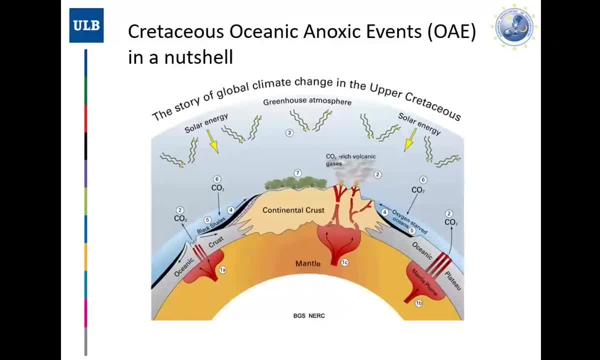 ocean to degrade this organic material and thereby deplete the oxygen in the ocean. so we are in a much warmer climate, so oxygen uptake is already reduced because the warmer waters contain less oxygen than colder waters and there's an enhanced consumption. so turning 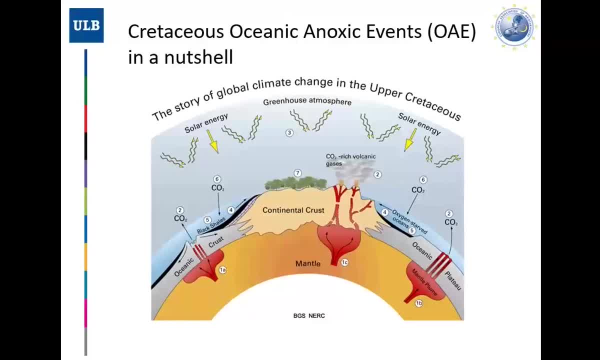 the ocean anoxic, and then this anoxic environment. with this increased productivity, you have a higher deposition of organic material. you're forming these big shales, you're burning this organic carbon, thereby terminating this event, cooling down the climate and the Earth. 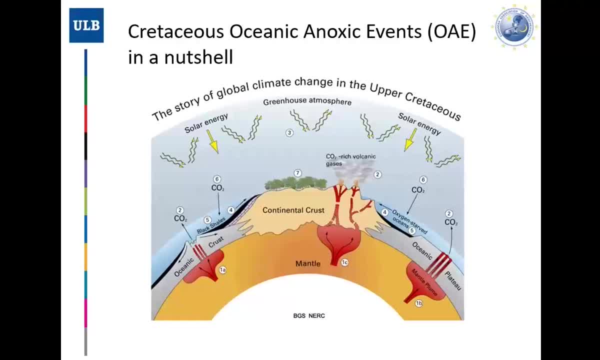 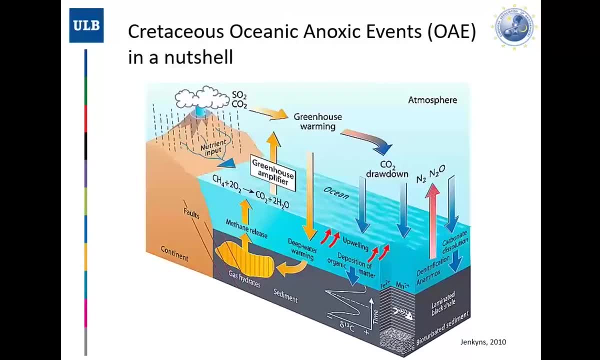 system returns to a much more comfortable state. So that's what we think happened. This comes with a lot of geochemical changes. so here you can see the same: increased greenhouse gases in the atmosphere. we have an increased nutrient input. Some people are doing something else. 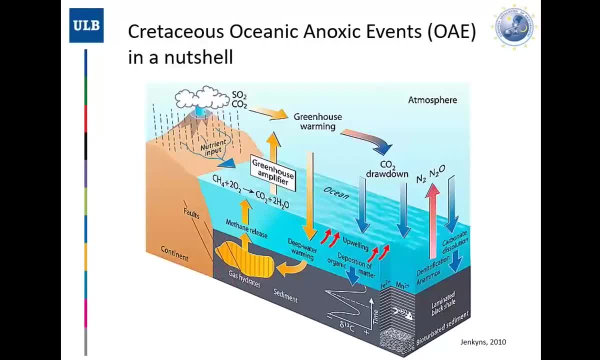 Some people are doing something else In some ways. definitely, there's evidence for gas hydrate release, so this is a further climate amplifier. so you have a warm climate. you destabilize the gas hydrates in the marine sediments. they release methane, which is a very powerful greenhouse gas, further amplifying. 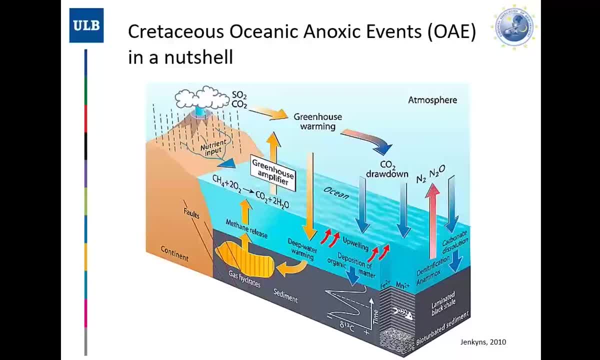 this greenhouse climate. you have this upwelling, this reduced this increased productivity. the deposition of the shales was a characteristic carbon excursion. You have the fixing of iron and manganese minerals in the sediment. the deposition of these really laminated black shales in these unoxygenated waters increased denitrification. 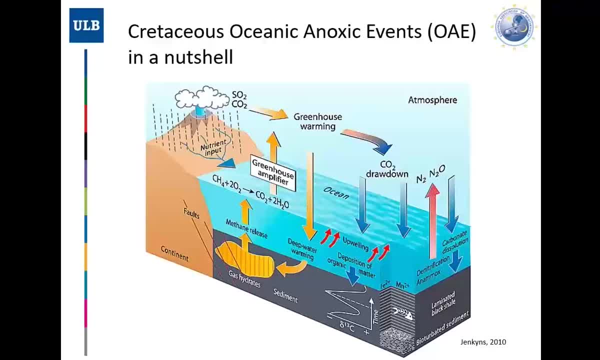 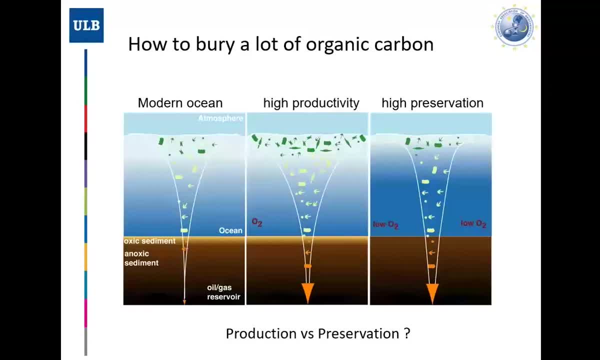 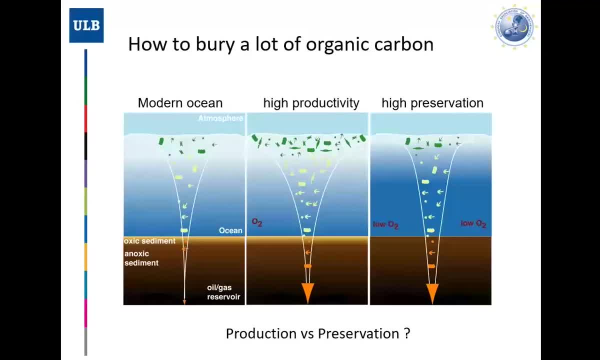 or is it high reservation? So there are these two ways. This is the modern day ocean. we produce hydro-plankton organisms fix carbon in the surface ocean. once they die, they sink through the ocean. they get degraded, this frogatic material. 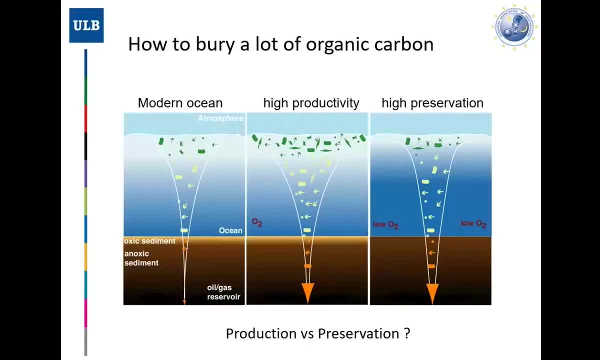 they die gets degraded on its way down by microbes. some of it reaches the sediments, gets buried in the sediment, gets further degraded by microbes and ultimately, only a tiny, tiny fraction what gets exported from the surface ocean gets ultimately buried in the ocean, in the deep 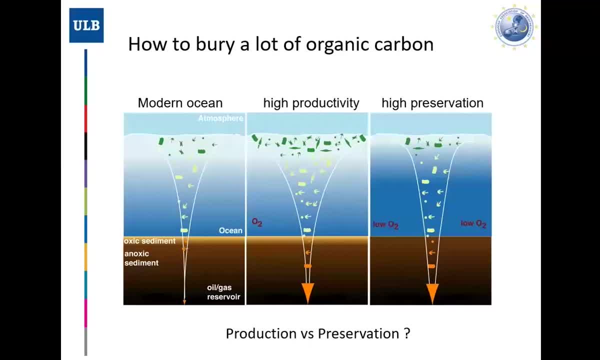 sediment. That fraction is very important because it controls a lot of things, among which, for instance, the concentration of oxygen in our atmosphere. but what we know is during the Cretaceous anoxic events, this fraction was significantly larger. So there are two ways, so you can either. 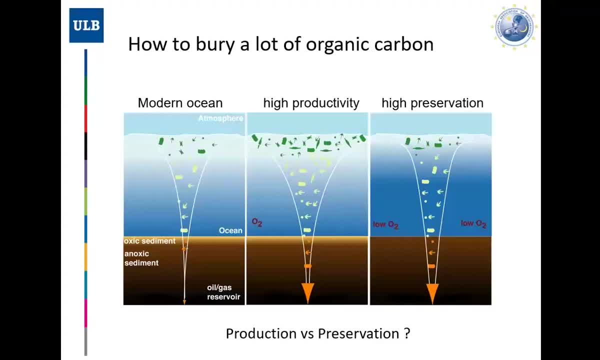 just increase the input and thereby increasing the output as well, the burial flux, or you can increase the preservation, so decrease the microbial consumption of this organic material as it travels through the ocean sediment system and thereby increasing burial flux. We know that there was. 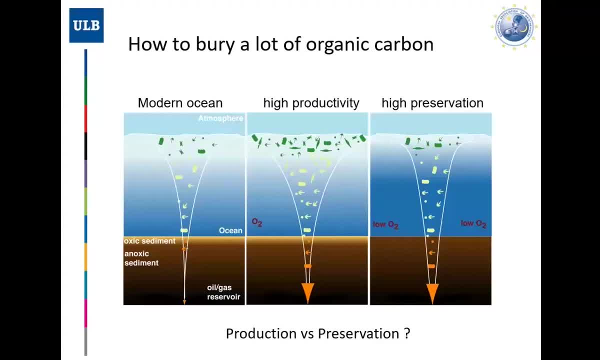 a high productivity. that's likely a high preservation as well, because in anoxic environments often organic material gets degraded much slower. so probably an end supply. but we have no real handle about what's the importance of these two processes and which one played which role in starting the recovery from this away. 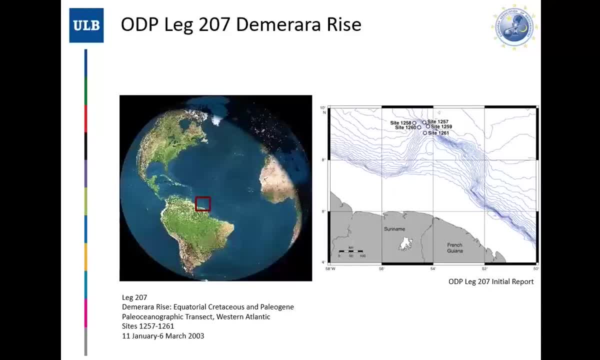 Luckily there's an ocean drilling program. This is a beautiful record and here on this ODP lake side 207, the Demerana rise, which was drilled in the early 2000s here just off the coast of Suriname. It's an oceanic plateau. there are five. 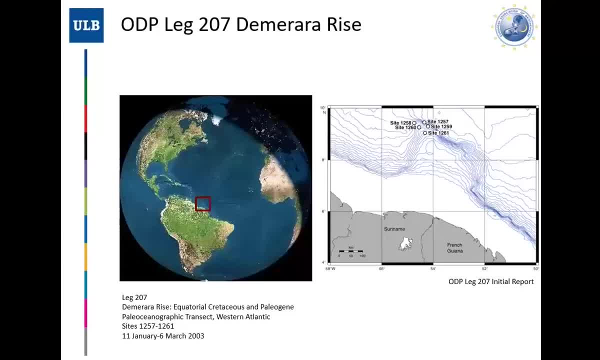 sites that are built here on the northern edge of this oceanic plateau, a few hundred meters of the sediment, and at all of these sites you'll find extensive um rotation, lake mutations, black shales from away too. so here you see a core photo. you see the black shell. that's an overlying. 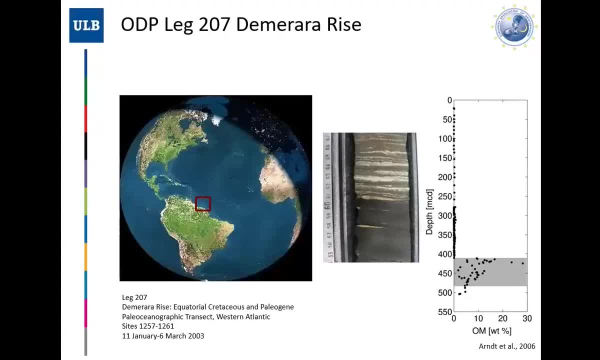 sediment. that's one example. that's also science. 1258 i showed before. so you have this extensive layer of organic rich material here, around 500, 400 meters down in the sediment. this organic metal content is up to 30 weight per set, which is quite a lot in normal marine settlements. 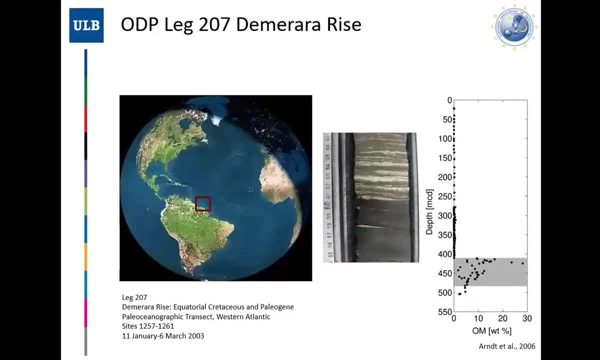 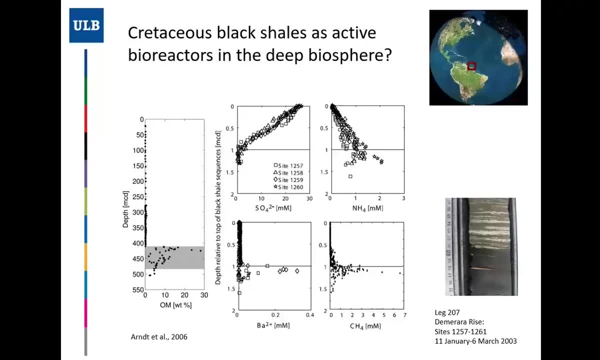 it's definitely always less than one way to set an unnecessary contribution. um, if you look at the pool water- so these are these waters that are in the core spaces between the grains- you can analyze their geochemical signatures. so what we see here. so here again we see this sequence from this one side. these are forwarding profiles from all the sides, and 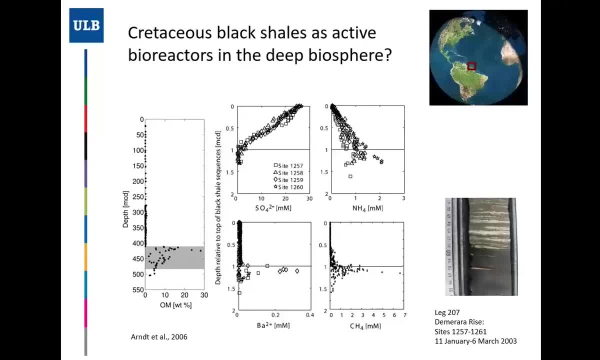 this is a little difficult to read, so here the depth scale is always normalized to the top of this black sharing layer at the side. so there are different, slightly different depths at the side, so there's some sites that are a little bit shallower. in some sense this one is one of the fatigue responses. 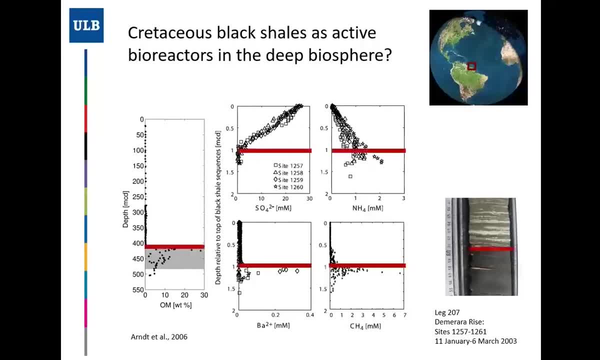 so here one: this line is always the top of the shells and what we can observe, that all of these sites are like very similar patterns in certain uh geochemical species. so what we see is linear degrees of sulfate from normal sea water values down here to the top of. 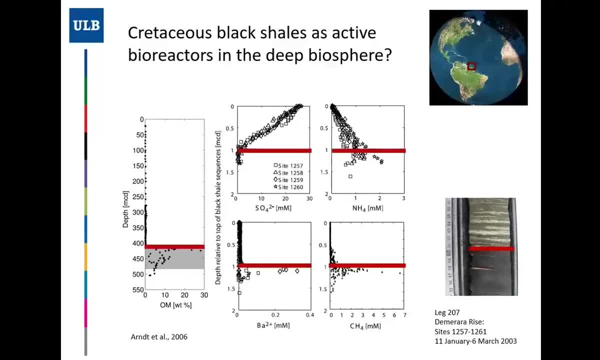 the black shares very, very low values. um same time we see an accumulation of ammonium um diffusing back up here to the sea floor to normal seafloor values uh. we see uh a kind of indications of methane production down here in this black shell layer um, and then subsequently we increase it to. 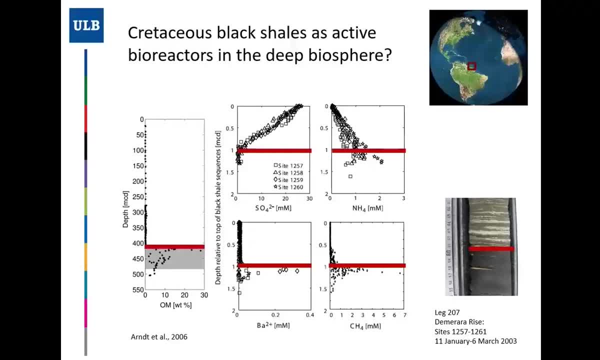 a certain extent and, uh, we can see that it has a lowerк, a concentration on the top of these black shea layers and accumulation of dissolved area in this layer and then you get a decrease of these concentrations on top. So, based on these profiles that we're having, there's very, very strong evidence that there 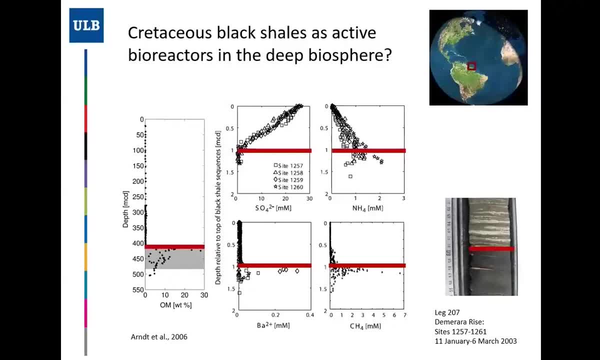 is something going on in these black shea layers And I still find that, even after this time, after all of this time, which is almost 20 years, I still find this absolutely mind-blowing. There is a hundred million year old layer of organic rich material that is growing really. 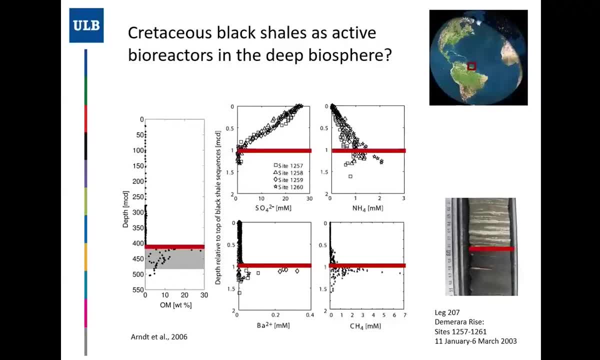 really deep down in the sediment and it looks like there are still microbes that are degrading this organic material, consuming sulfate, producing methane and producing ammonia. So this is why it's amazing. So this, based on this we know, and this is also one of the achievements of the 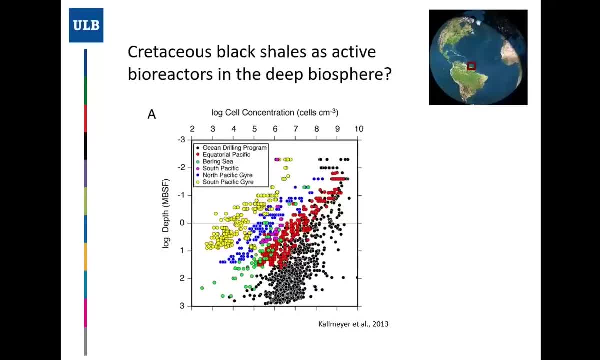 ocean drilling program. it's like we start to know a lot about what we call the deep biosphere. so it's a biosphere that lifts down very deep in the sediment and we know as you go deeper in the sediment. so this is a mock scale, this is a depth in the sediment, so we would be around this range. 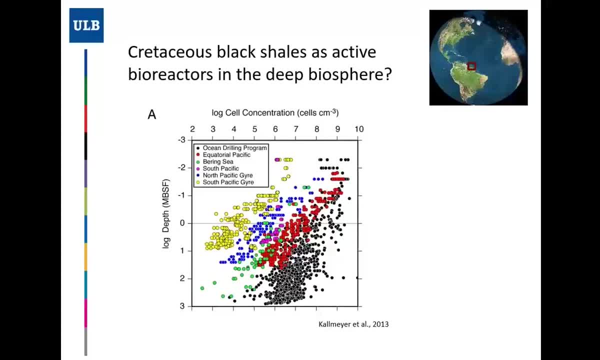 here. So this is a number of cells. so we know that there's a very rapid decrease in the microbial cells. so we know that this is a very extreme environment. So you have microbes that live deep down there that are using organic material that was produced a hundred million. 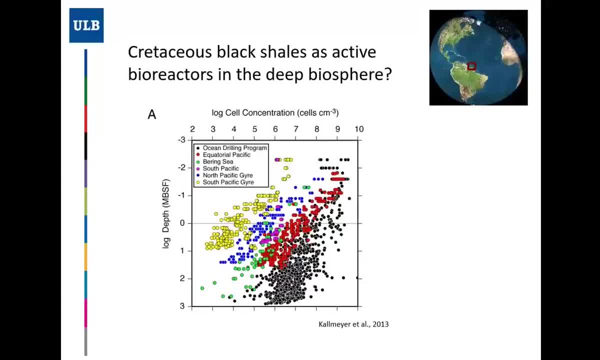 years ago in an ocean that was completely different from what our modern ocean looks like, and they are still degrading this material under this really, really hard conditions, So very, very far away from any oxygen. there's no oxygen. that counts down. 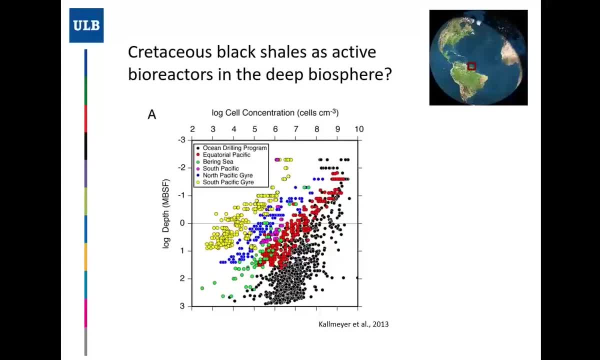 or any powerful terminal electron acceptance and really just using either sulfate reduction or methanogenesis or very little energy gain for them to maintain themselves. So this was our hypothesis. So it's a question: are these glutaceous flex shales active bioreactors? 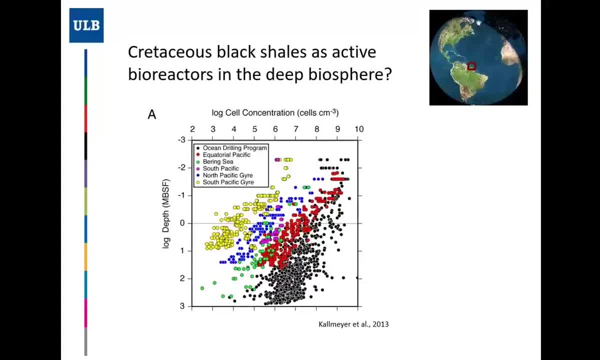 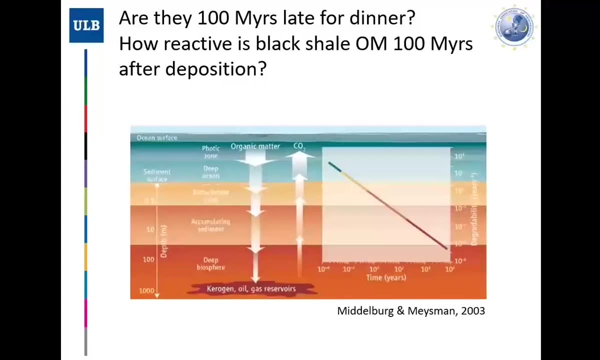 in the deep biosphere Is there Active microbial degradation so you can't incubate that? people have tried it. it doesn't really, because the rates are so low that you can't really see anything. so how do we find this out? What we also know is like based on previous studies: 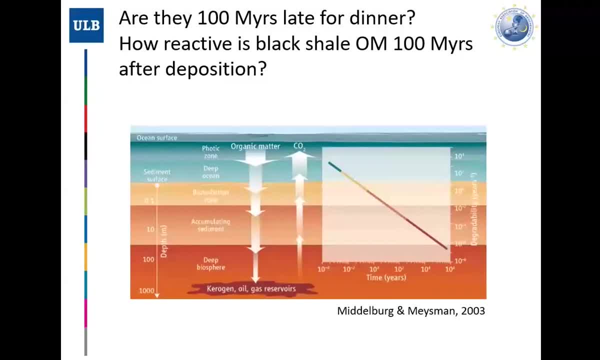 so this is a compilation and you don't see the data points here, because that's a really nice conceptual figure. but this line obviously is fitted to data points, this combination of a lot of incubation experiments and other methods of determining the reactivity of this organic material as a function of age And as you can see, 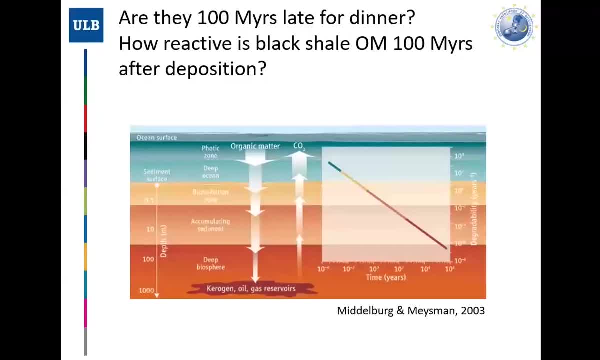 this is really nicely fitting this vertical view. so obviously we have organic material being produced here, so it's very fresh, it gets degraded very rapidly, it has a high reactivity, it's very juicy, it's something the microbes can easily access and consume and as it sits, it's a 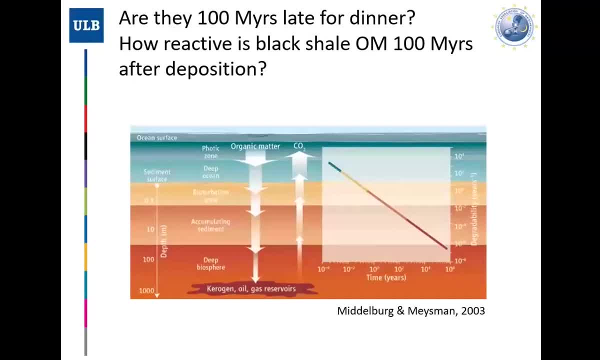 whole thing that goes down in the ocean and gets older. all the easy to degrade implements are already degraded, and after a really, really long time. so here we are: a thousand years, ten thousand years, you end up with something that is not that reactive, and that could be the range. 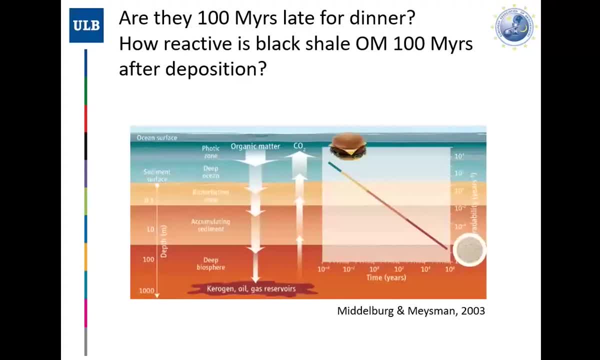 we are looking at, But I always like to think about it as like the burger and rice cake scale. so you have some very yummy food out there and some- um, eatable food, but maybe it wouldn't be your first choice if you would have a. 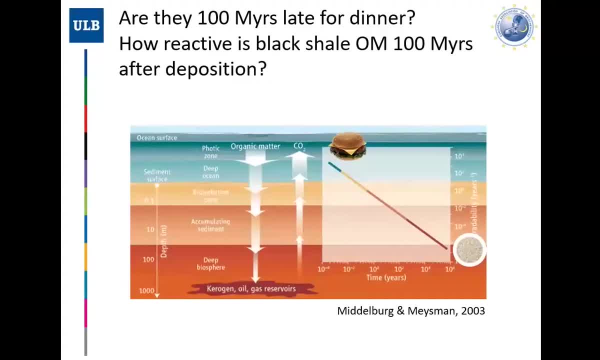 whole planet of foods to choose from. so it's really the question: where are we here in these black shales? um, do they fit this, this concept we have of the ocean? uh, do they lie completely somewhere, completely here? you see, the data is up to um a million years. yeah, that's a million years. 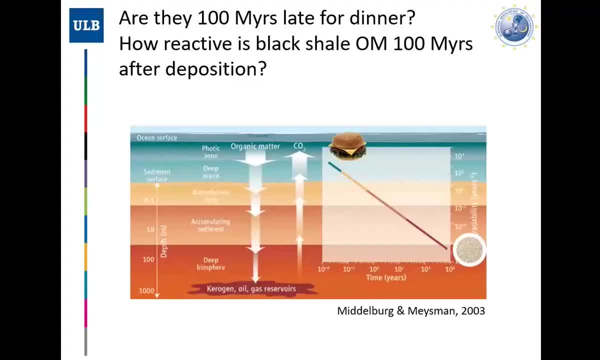 uh, the greatest potato spec shale would be like: uh, another two orders of magnitude and a million years. uh, down the line here, there. we didn't have any data from that. so how do we find this out? we can't incubate, um, we have the poor water observations. so that's the only information. 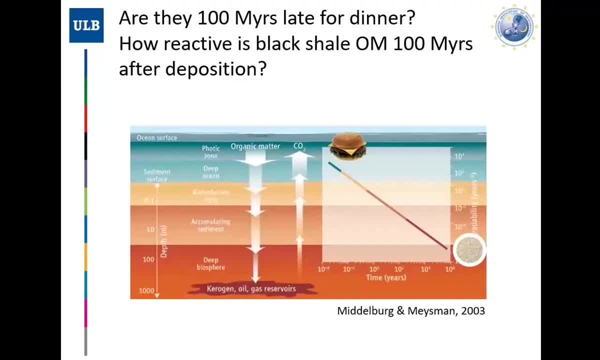 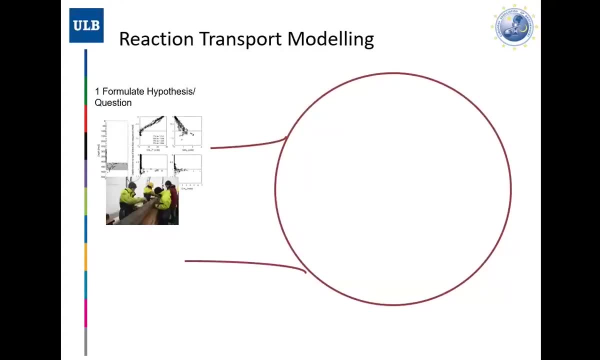 we have from which we could potentially extract quantitative information. so how do we do that? and so, uh, modeling, reaction transport modeling is a great tool, um, because it allows us to test hypothesis, but also to um formulate these research hypothesis and extract this quantitative information. so how does it work? i have my observations. you've seen us that were measured. 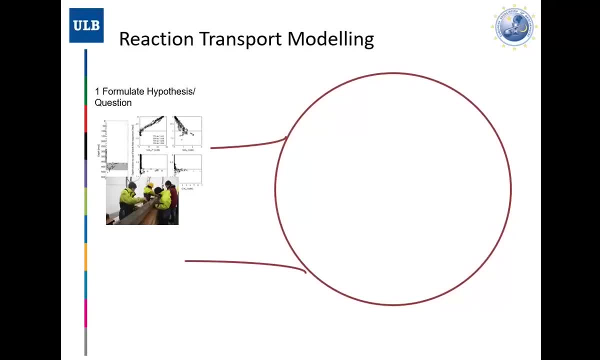 on board on the lab afterwards. and then i have my specific research question. i'm asking and i'm building a reaction transport model. so it's basically a model that simulates or that builds a virtual sediment column. so it simulates like the concentration profiles i'm observing here in my home and with this model. so i put this model. 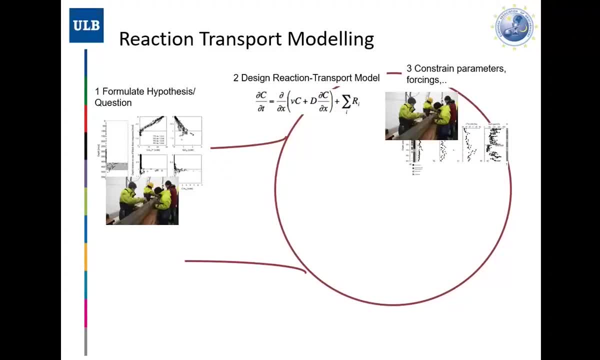 i constrain parameters, so all the reaction parameters but also diffusion, affection, forcing um conditions, um, i know what's happening, or i have to constrain somehow what's happening at the boundaries, bottom water concentrations, and then with this information i run um and then typically i compare the simulation results with the observations and if you do that circle one time. 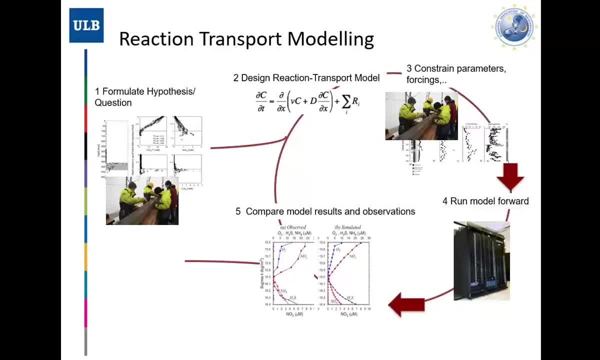 typically that doesn't fit. yeah, so it's. uh, it's very, very rare and almost never happens that your simulations fit the observations. it's because there's something you're missing out here or something you're missing here. so what you do? you go back. you go back either to the model or to the parameterization. 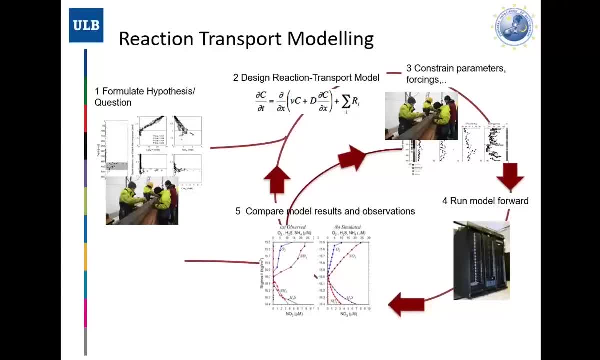 you have a look again, you say, okay, what am i missing? um, maybe there are certain parameters you don't know very well. so you've been testing other possibilities and you're on the model again and eventually you will get a good fit and that will give you an idea, um, of what's happening. 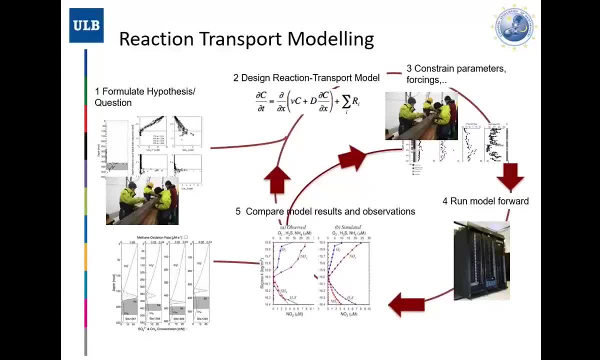 of rates that are happening down there, and this will give you quantitative information. now there could be obviously more than one possible solution to that, so you could have different assumptions. you could have different models with different parameters that fit the observations equally well, um, but it's typically in the very narrow range. 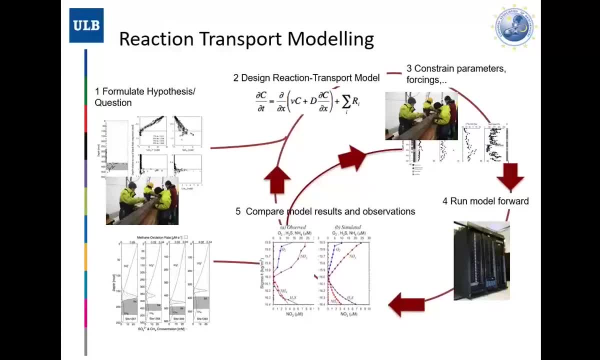 that's your uncertainty. um, very often you just have this one range of solutions that fits your observation, especially when you have the right one. so you have very comprehensive cool water and solid phase geochemical profiles, like you get, for instance, from otp cores. so they contain a lot of information. you have a lot of extra information. 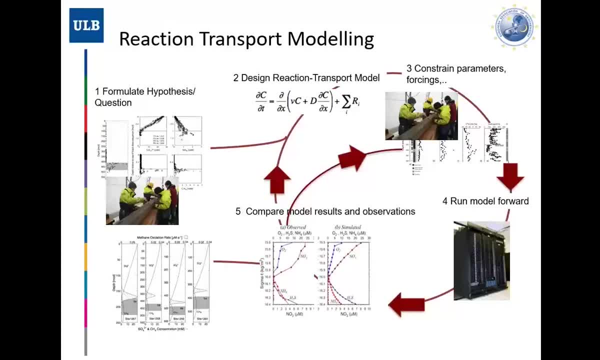 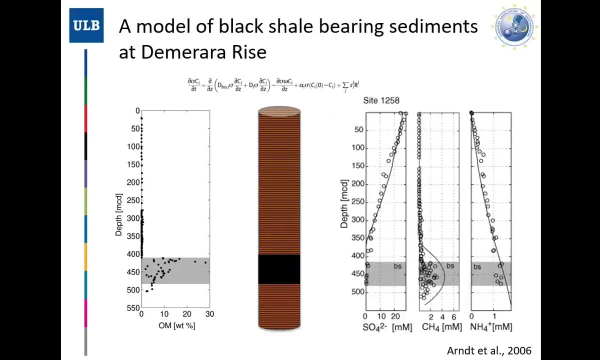 from the biostatic graphic rapid, for instance, and with all of this information, if we put all of this information in the model, you typically arrive at a very narrow range of parameters at the same screen. so that's what we did: uh, took the observations, built this virtual sediment pool with this. 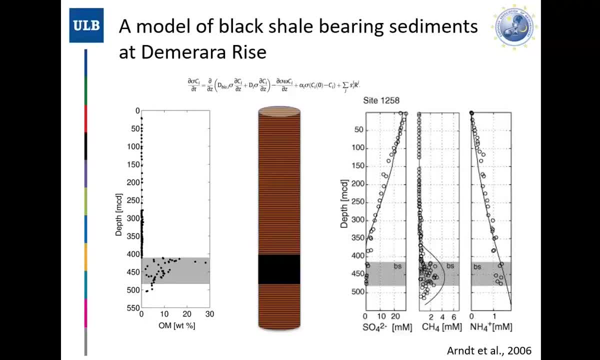 next layer here and then try to fit the pool control profile. so here is just the fitting results. from one side you can see that sulfate is the model result, the the line, the observations are the points, and what you can see is like it's, it's fitting. pretty well if you see this. 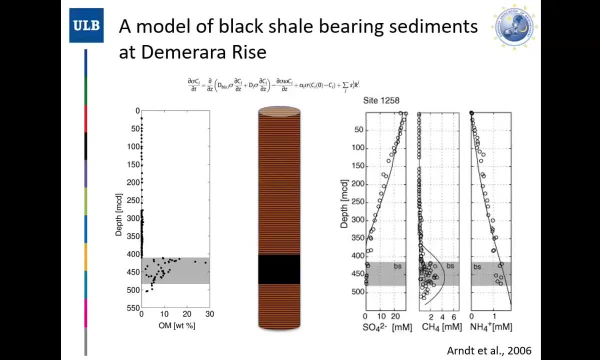 decrease in sulfate. um, you even resolve some of these little buildings which have to do with ferocity changes and changes and transport parameters. uh, methane concentration here is it's normal that the model predicts higher concentration, because these observations are not, uh, quantitative, they are only qualitative. anything else, uh, rapidly the absence, uh, so it's. 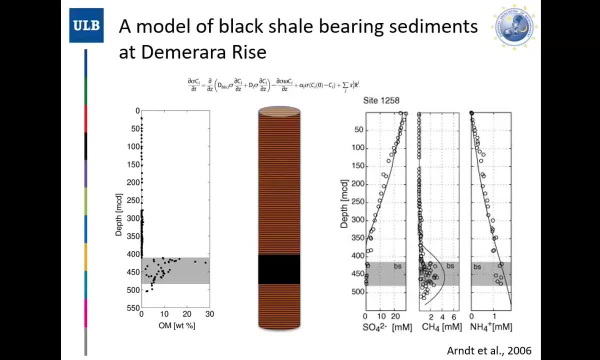 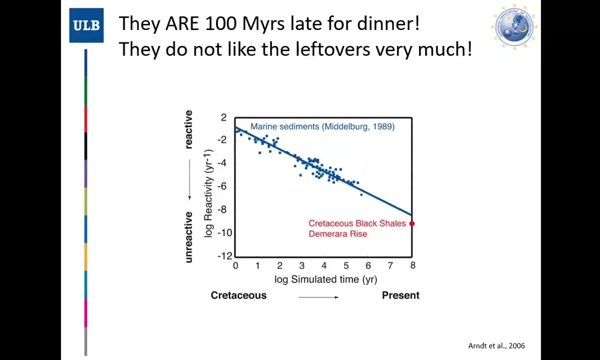 it's basically just indicating the presence for non-reliable concentrations, or, quickly, ammonium. pretty nice, fit and out of this. uh, so by fitting this we we get the parameter for the reactivity. we have a quantitative information for the reactivity of this organic material. so the the parameter says that fits best. the observations is basically here, so 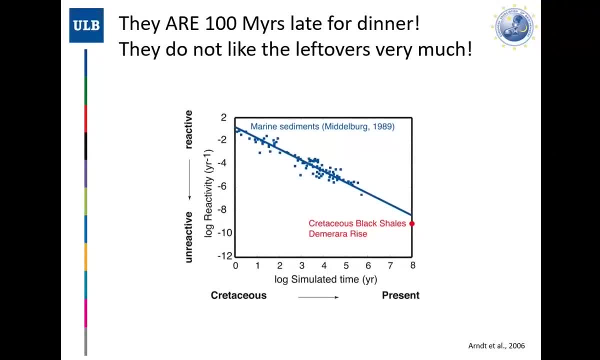 falls pretty well on this general trend. so what we see is like: yes, these microbes there are hundreds of million years old, so they are still degrading these um contagious black shales. it's just they are not very reactive. that's also something we expected. this is 100 million year old material. 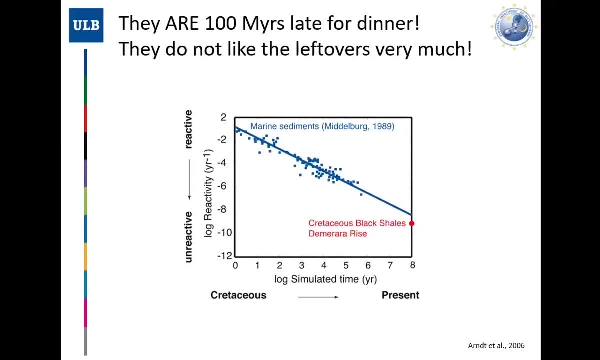 that has been degraded over 100 million years, um so likely the material that's left over, even though there is still lots really good proportionate. so some of these organic carbon components were 38 percent, but it's quite significant. uh, it's, it's very unreactive. 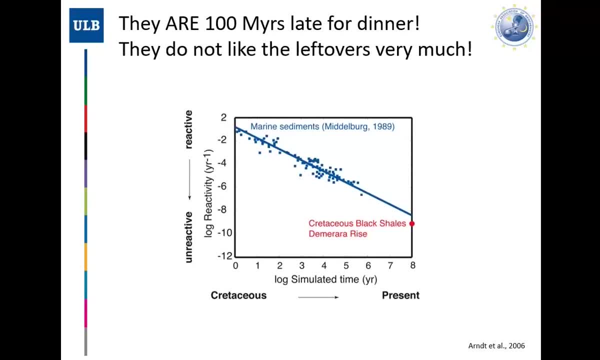 but it still doesn't tell me anything. so this is a now situation, so this is just saying this is what's happening right now in the deep ocean, in the deep sediment, uh, but it's not telling me what happened back in the cretaceous at the oau ocean, in the oau ocean. 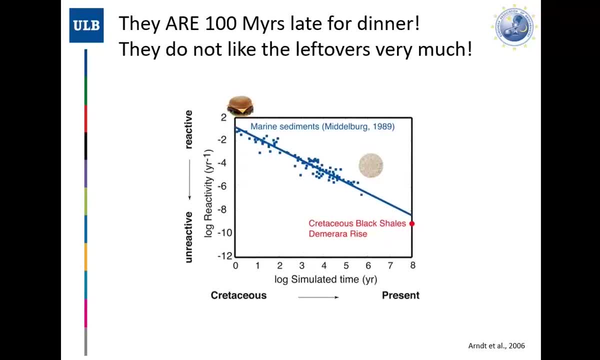 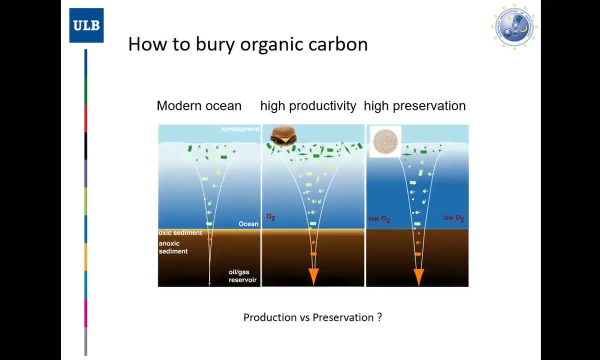 were these cretaceous leg shales rather here in the normal, like burger space, or were there already rice cakes? so otherwise it's like: was it the productivity there was tiringness, which would indicate this is the normal world, or were they already quite unreactive and this is why we see such high organic carbon concentrations? so it's not answering this. 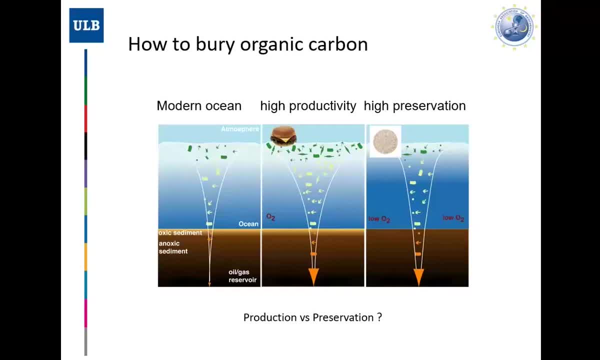 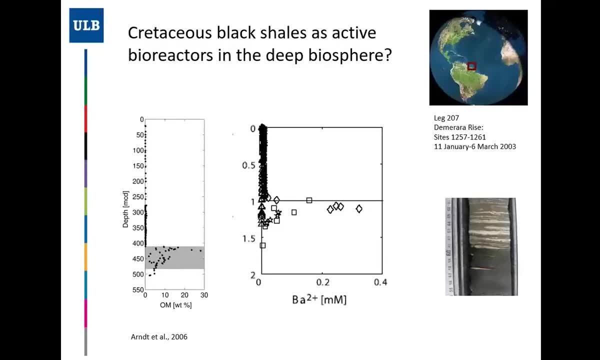 question. we don't have an information about this, so how can we answer this question? so i'm doing this work, what we've seen, so i'll take you back to the border profiles. where we've seen on the border profiles there's also an accumulation of organic carbon that's already quite reactive. so 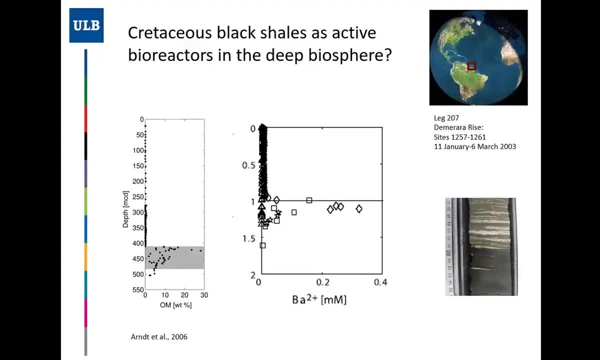 we can see that there's an accumulation of organic carbon down in the flexion layer and that kind of disappears on the top of the flexion. now that is something that's not really difficult to figure out. what's happening here, because that's happening in a lot of other. 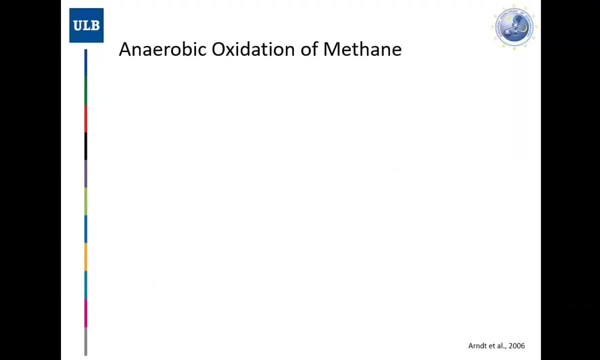 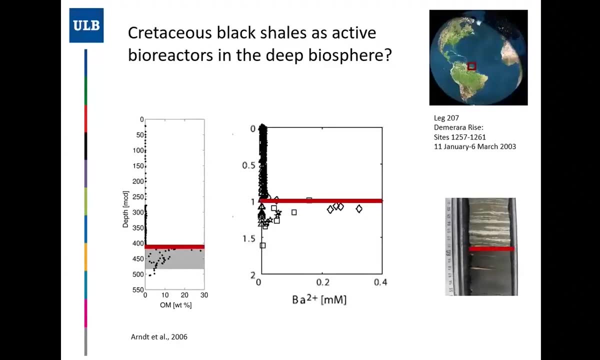 sediments as well. um, what we see here is is basically it's it's like there is biogenic barite, that is um always enriched in organic matter, rich layers. it's used as a party proxy for highly productivity. so if you have a lot of organic matter, it's very likely that you have. 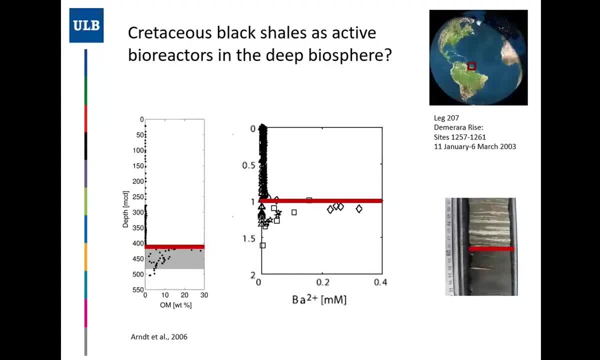 one biogenic bear right in nervous. and this barrier is actually thermodynamically not super stable as soon as the sulfate is, uh, depleted in the pool, as it starts dissolving- and that's what we see here- there's no um sulfate ground in the back shells, um, so the barrier is dissolving. it's. 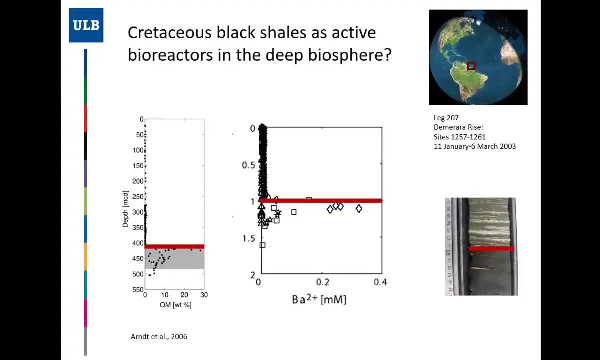 diffusing up full and as it meets that sulfate it's gone. so the sulfate that you're looking at is diffusing from- uh, the seafloor down. it re-precipitates as autogenic values. so as soon as the board has become over saturated, again with respect to their right, there is re-precipitation. 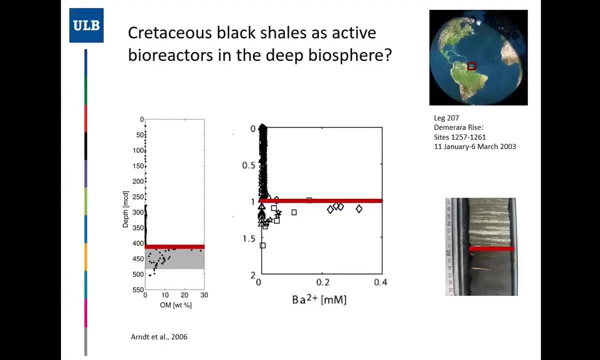 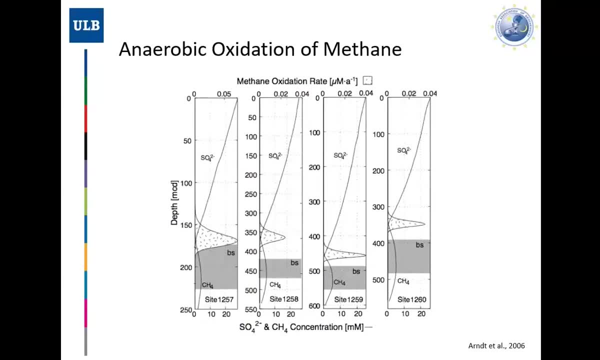 of their life and these autogenic fronts is something that we see very often and we see very often associated to the anaerobic oxidation of movement. so when we see all these courses of the previous um results from uh four sites, it's like you have like shea lake. 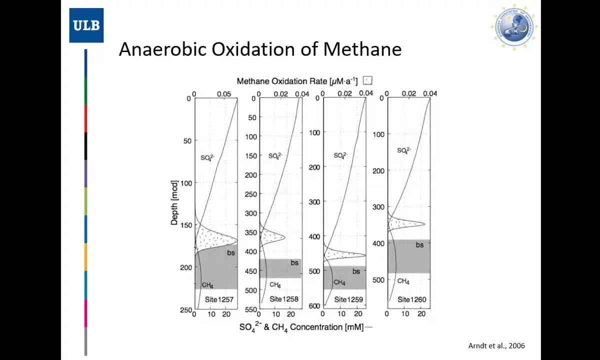 so you have sulfate diffusing down from the seafloor um and being consumed by the methane that's produced in the black shells, that's fusing upwards, and they have microbes that then oxidize that methane with the help of sulfates to co2, and that's always here at the top of the flexion layer. 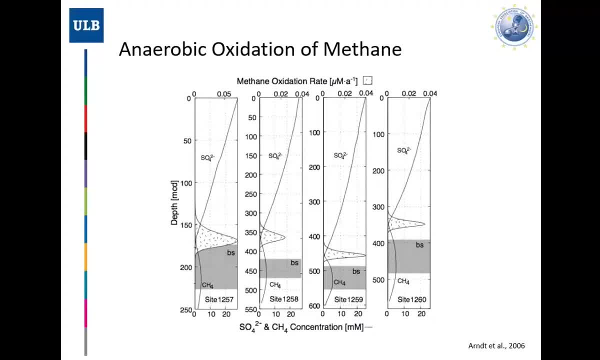 so that was our hypothesis. so you have like the sulfate equation in the black shells that's dissolving the biogenic barite, um barrel dissolves upwards and precipitates probably in this aom science. yeah, so the idea was like, well, if we would have a very detailed record of barry just on top of these black shale. 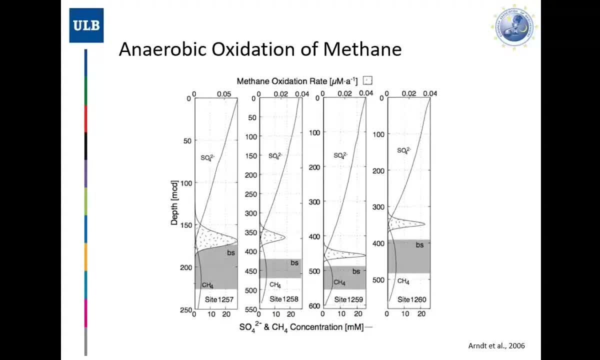 layers. um, maybe we could reconstruct the movement of this sulfate methane transition fronts and through that we could reconstruct the methane production in this black shale and maybe with this information, that would give us some information of how reactive that material was over the past hundred years. back at that time it didn't happen. so what we did? 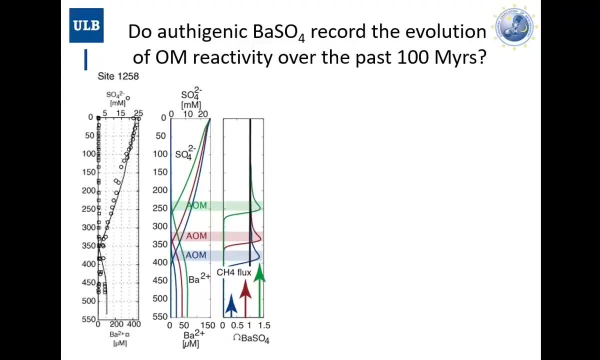 it's like: ah yes, it's the same. um, also, what we've seen in this is like that: um, the sulfide methane transition front is actually quite sensitive to the methane flux that's coming down from the black shale. so if you just double the nuclear flux, you shift that ground by 50. 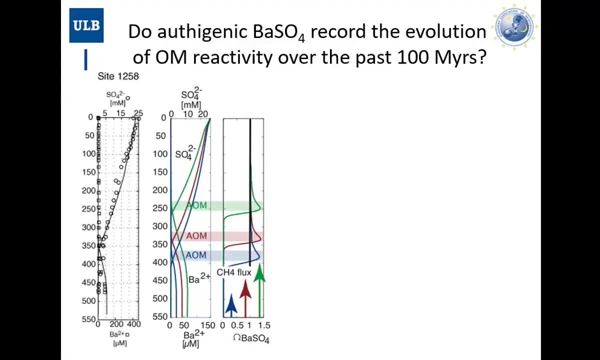 meters in the sediment record, so it's a really really good indicator of how much methane is coming from the black shale. so therefore it could be a really good indicator of this smtz migration over the past hundred years. so that's what we tried. it's. it's a little bit of a crazy. 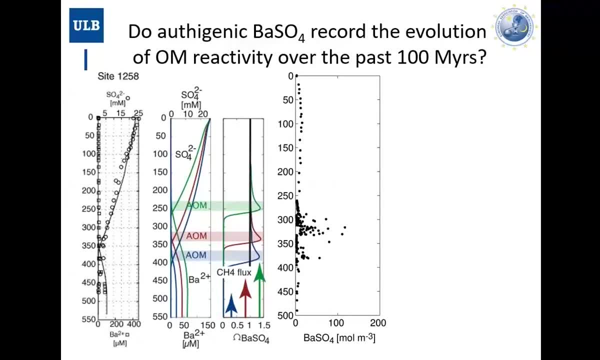 idea. but you know, when you're young, you think like you know it all and you can do it. and uh, interestingly. so we went back to the pool and we found that there was a pooling of mine- sample of this layer just on top of the black shade in. 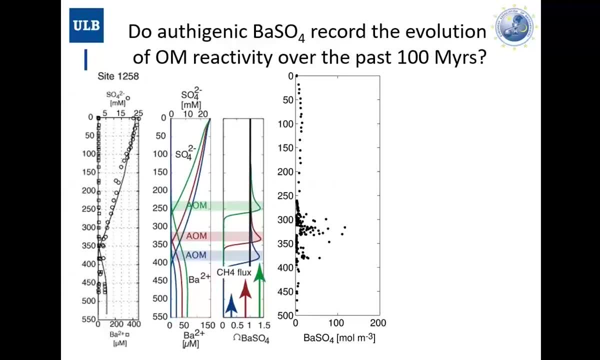 high resolution and we found this bear ice profile, um, and then somebody did a super isotope analysis on this and you can really see that these are also, uh, autogenic precipitates. yes, so this is an autogenic right record. it's. it's not a paleo right back, it's a secondary signal. it's not balanced. 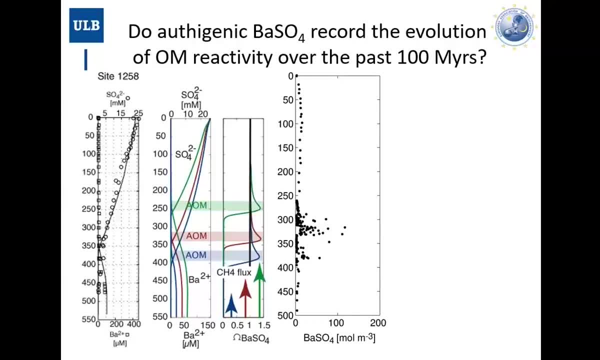 So the idea was like: okay, if we manage to like, reconstruct or run a model over 100 million years with the conditions of deposition at this side, and manage to reconstruct this record, then we have learned something about the methane flux out of the black shale and its reactivity. 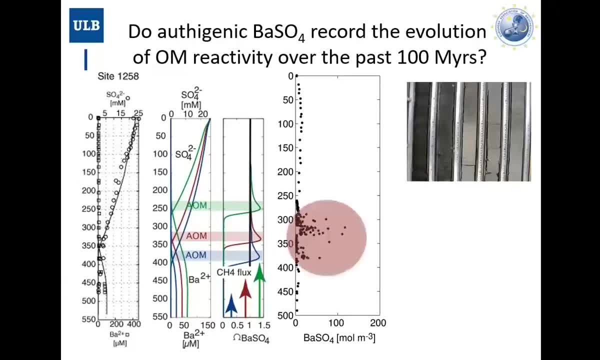 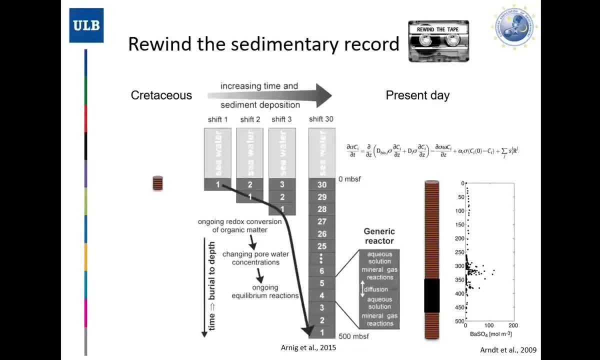 of the organic material. So that's what we did: to reconstruct it and learn something about the rotatious environment. So you take the model we built and then it's kind of well. you're probably all a little bit too young. 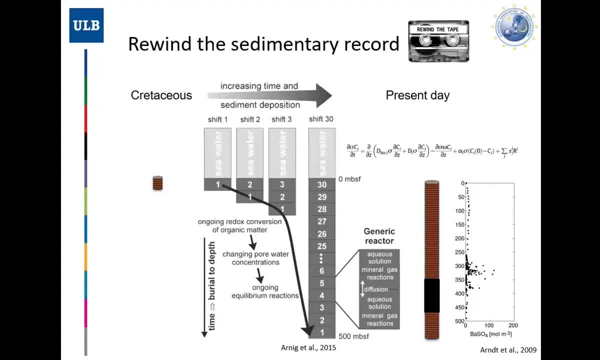 This is a tape And you know, it's like when you listen to a tape it's like you turn it around or you have to like rewind it. So this is kind of like rewinding the sedimentary record. 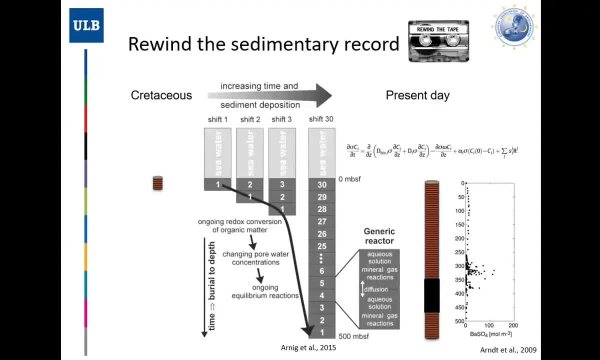 So this is today. we want to go back at the time where this was just deposited. So we spin back the model and then run it forward and let it produce ferrite. And we do that many, many, many, many times with different assumptions about the reactivity. 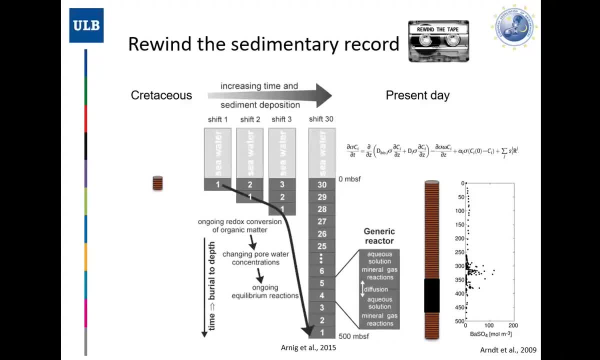 of this organic matter on the black shale. In all the information about sedimentation rates, we have sulfate concentration in bottom waters over the past 100 million years, Which is obviously very, very coarse information. It's not that we have a yearly record of sedimentation rates. 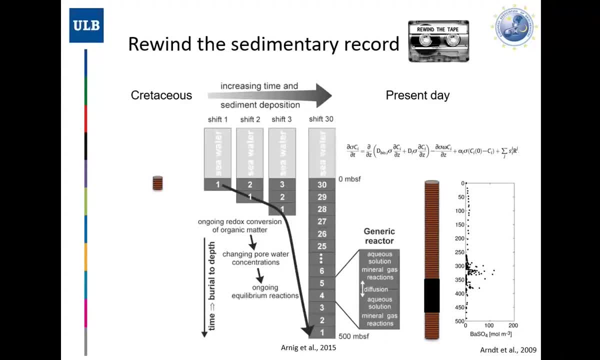 So we have many years of sedimentation rates for longer geological times, And we try to find the solutions that come close to this record And that tells us something about how reactive this material was. And so that's what I did, over a lot of iterations, and, interestingly, this was something I didn't expect. 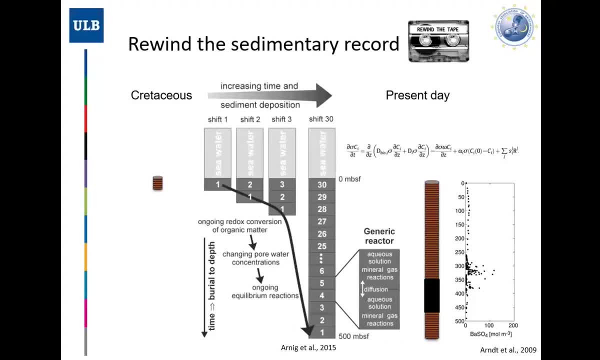 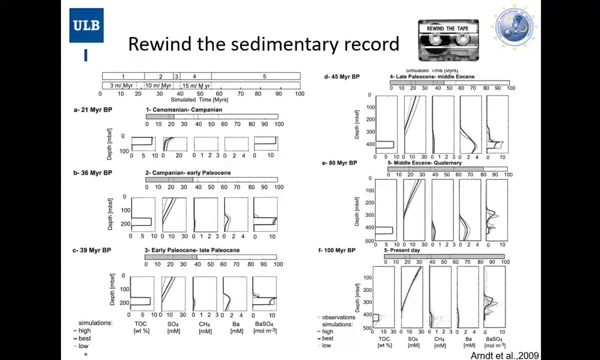 there was only like a very narrow range of solutions. Yes, something that looks like this. So here are the results. So you see three different lines, therefore three different sulfate concentrations in the ocean, because sulfate concentration has changed from the Cretaceous to the present and there are uncertainties of that in the reconstruction. 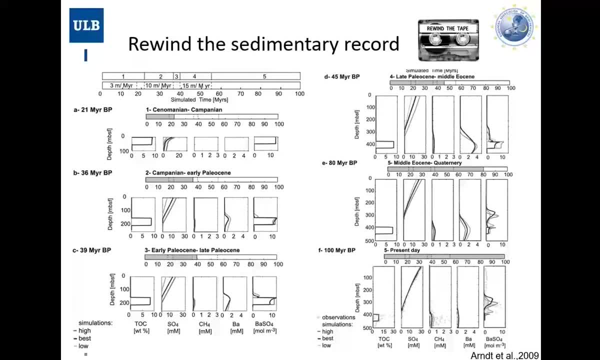 So they kind of give the envelope of these uncertainties. It's a pretty important factor. And then we have linear sedimentation rates for different periods that were determined from the H-model for these cores, and what you can see is like roughly similar periods. This is obviously. 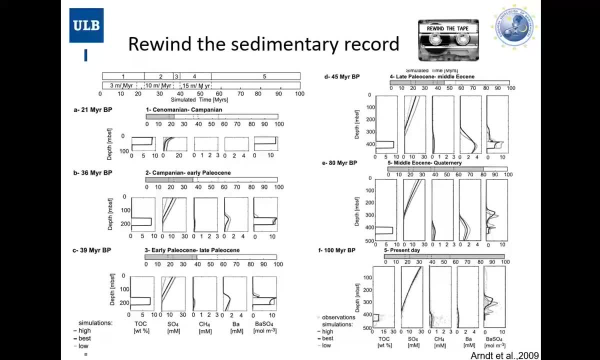 also a very stark simplification because obviously the sedimentation rate is not three meters per million years, it's almost 20 million years. It probably varied quite a bit, but this is just to be sure. So this is just to get the general picture and we have some important. 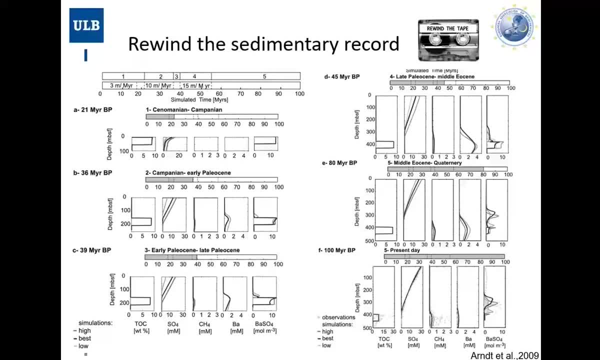 hierarchies that play an important role for the autogenic mineral precipitation because they allow these fronts to form. So if we get these right, we already got a good handle of the record. So what you can see is like you have the next picture. this just after the deposition of the 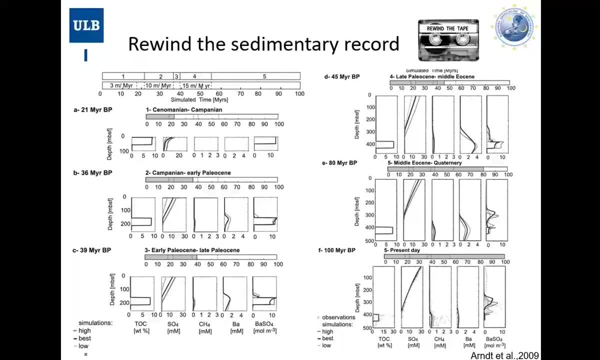 Cretaceous material and it gets buried down over the next few times of the reconstruction. So you can see that the Cretaceous material tends to form over the years. buried down you have, like the barite dissolving and here's the biogenic barite. you have an autogenic one forming here. 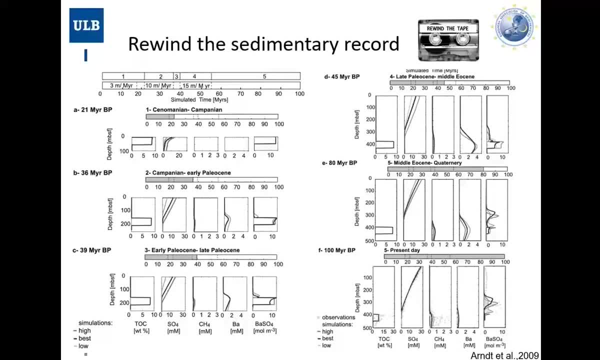 then you have thriller sedimentation that smears out. so because the sediment is buried and the sulphate methane transition zone is moving upwards continuously, you have like this record that moves up. then you have a hiatus. you have a big one that's forming here. 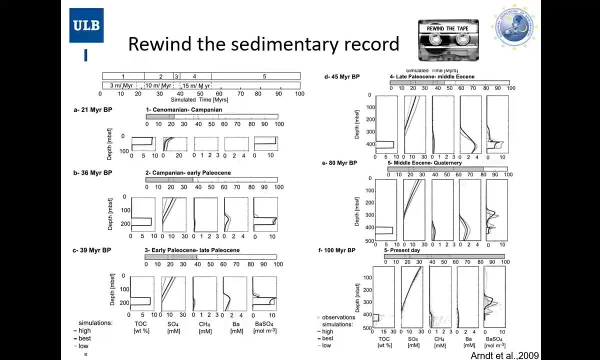 and then moving down again, the present one that's forming here, And you can see, you can really reproduce these two peaks, So it's a paleo peak. then the front that forms through the hiatus, while this early front is dissolving and then re-precipitating another autogenic barite front. 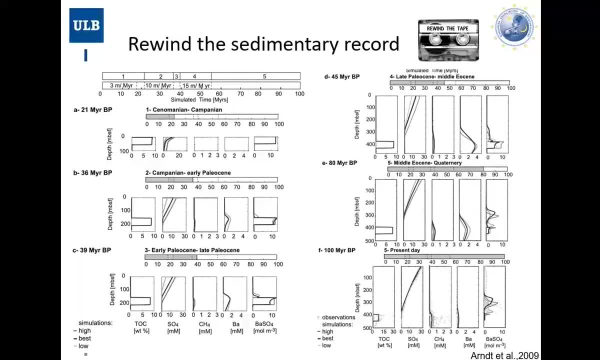 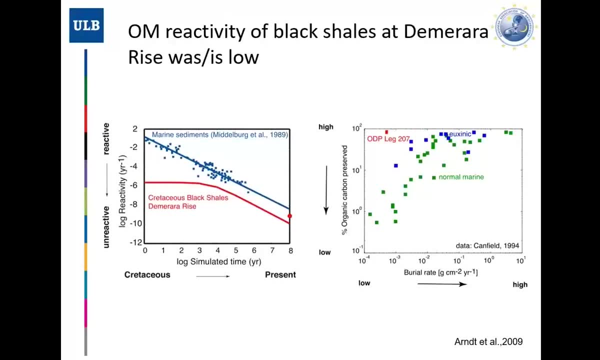 at close to present day conditions. And when you do that, it's only a narrow range of organic metal reactivities that gives you this distribution, and this is the reconstructions of organic metal reactivities in these Cretaceous peaks shape. So what you can see is like they were already quite unreactive even at the time. 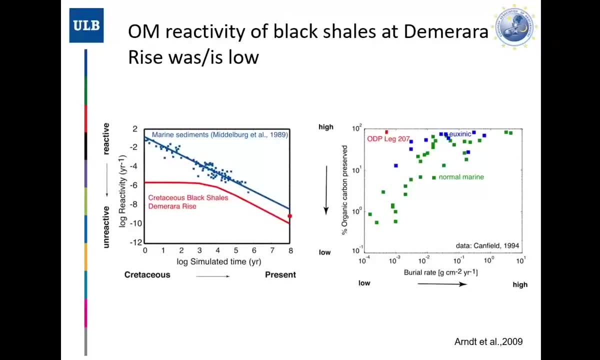 of deposition. So typically you would expect at the time of deposition something in this range, so normal reactivity of marine organic material. but there were already orders of magnitude less reactive than this early material and then also less reactive Throughout time, And that indicates that there was a higher preservation of this organic material. 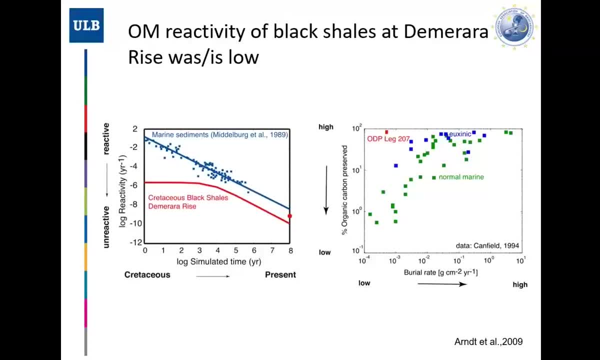 in these lectures and what you would normally observe in a normal environment. That fits really well, but because what we know is like during these times in the Cretaceous, the equatorial Atlantic, so this was a time when the Atlantic was in the process of opening and the equatorial 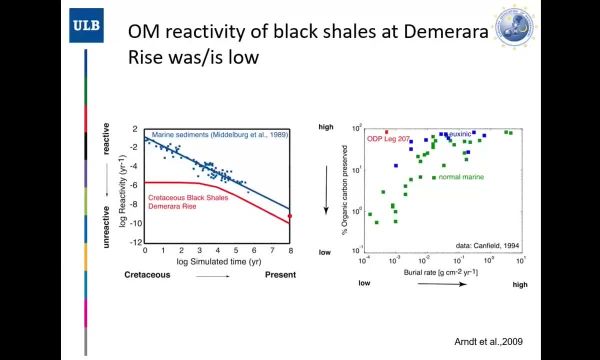 Atlantic was very unoxic and very hypoxic, so there was a free sulfide And, as you can see here, in this combination, uh, we don't can feel um. in like scenic environments, uh, you have a higher preservation. 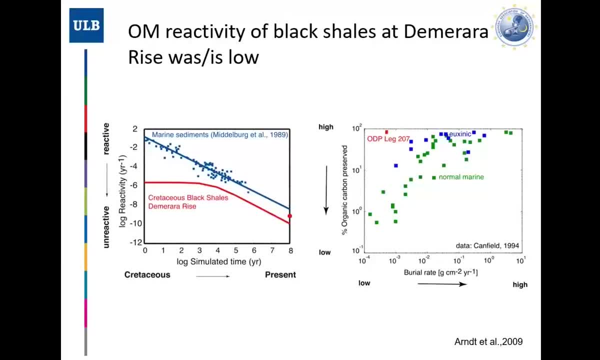 Uh, so the organic material is recurrently preserved, not degraded. That fits really well to this uh, Cretaceous peak shape and we determine preservation efficiencies of around 80%, which also makes sense, because if you nowadays find 38% um in an organic 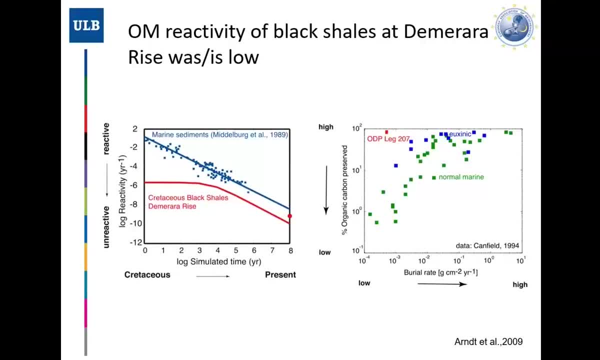 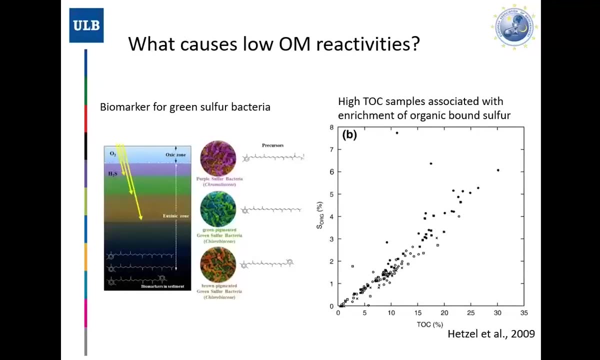 which deposits it's: uh, it's very unlikely that you have a more degradation, because that would mean you would have a- yeah, but in the worst case, of a hundred percent, which is unrealistic- um concentration of organic carbon. So what causes this low organic metal reactivity? 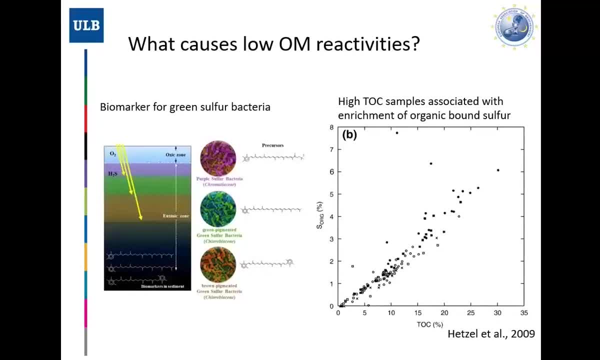 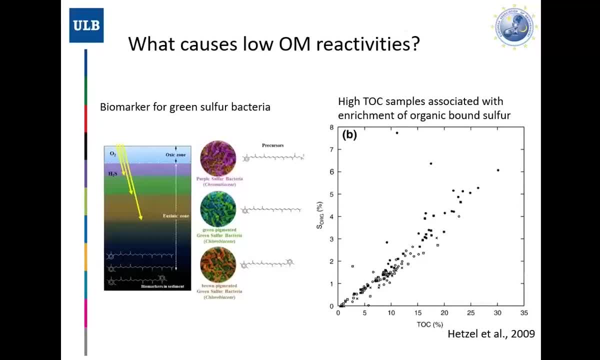 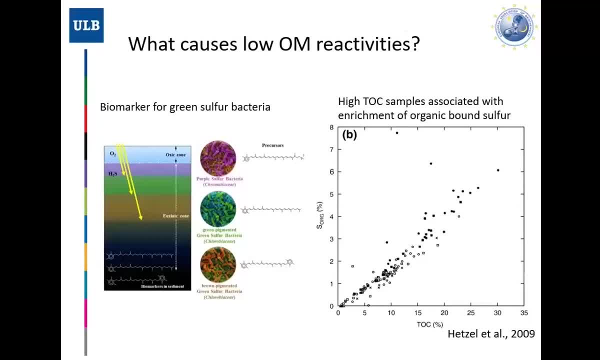 So and again, luckily this is an ODP site, so there's a lot of data coming out and there are a lot of people working on different aspects. So we have the organic geochemists who find biologist stoppable green sulfur bacteria. so there's a material that the photic zone 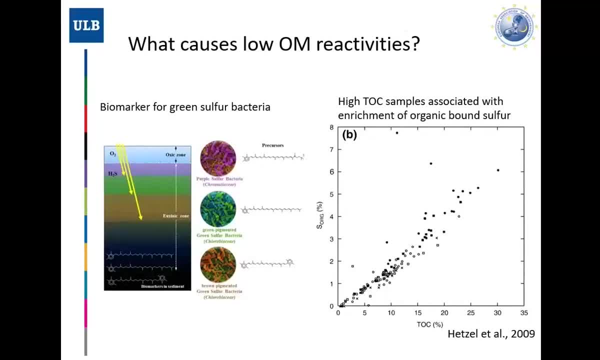 which indicates that there were photic zone in Yuxin yang so in very, very scenic environment. So that fits well. What we also found find is that there is a link between organic carbon contents and sulfur in this organic material. So what happens is like in these sulfide-rich environments, the organic material 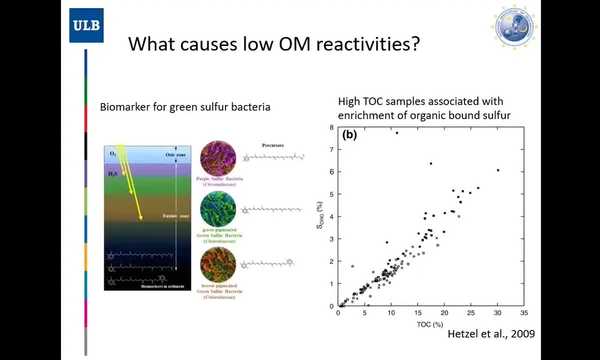 can react with this sulfur and can form very stable bonds that are very, very difficult to break, And so our hypothesis is that, like in this fuchsia environment, this organic carbon has been made less reactive by the sulfurization of the organic matter in this contagious motion. 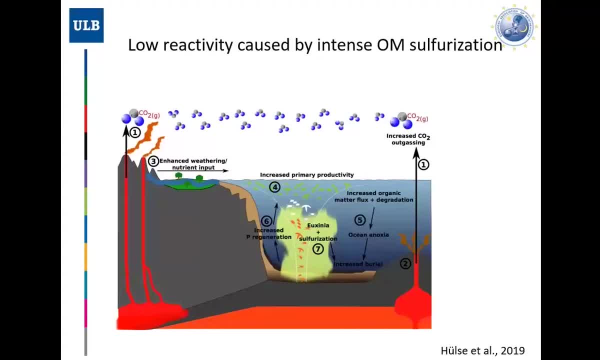 So sulfurization, so this is how I think it works. So you have the increased climate productivity, you make the ocean non-oxic, you make it very sulfidic. you have- we've seen you up here into the project zone- a lot of the sulfide in the water column. 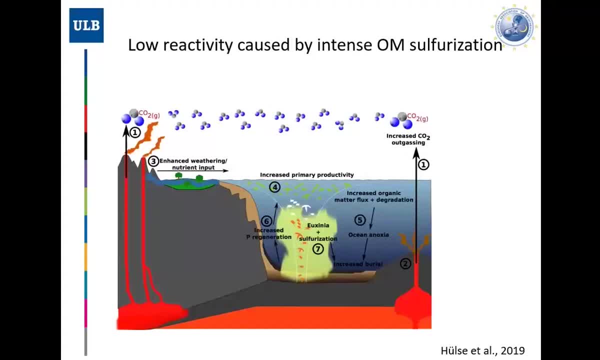 and then you have the sulfurization. Back at that time what we knew about sulfurization of organic matter was that it's a rather slow process. that happens in the sediment in really long time scales via condensation reactions or time scales of a few thousand years. So slow process which 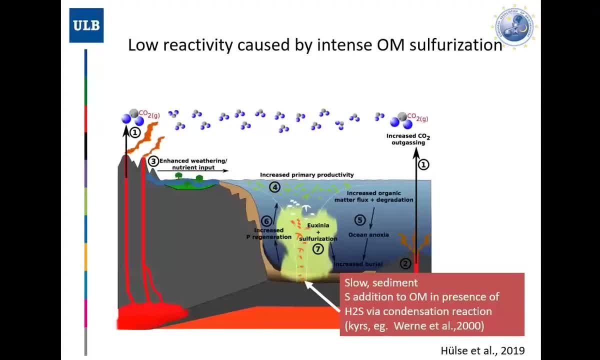 is helping the preservation of the organic material that's buried there but wouldn't necessarily have a direct climate. But then a few years later, a few decades later, in Carriaco basin there was some work published about fast water color sulfurization. So there a lot of the 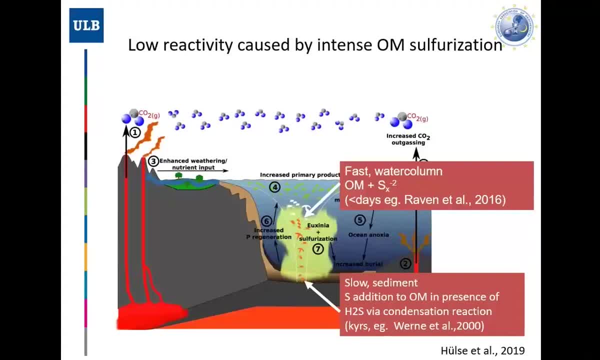 organic material that sinks in this non-oxidic basin is sulfur And that which is ideal in a present moment. and whether it is evaporated, even before it reaches the sediment And organic material, it is sulfurized and makes up the big portion of organic material that's buried in the sediment. So if that's happened in the water column, this will likely have an impact on the carbon cycle and on the relics conditions on the ож. So our question was like: well, if organic matter is, if it is subsctions into the ocean, under water, how important is it doing? 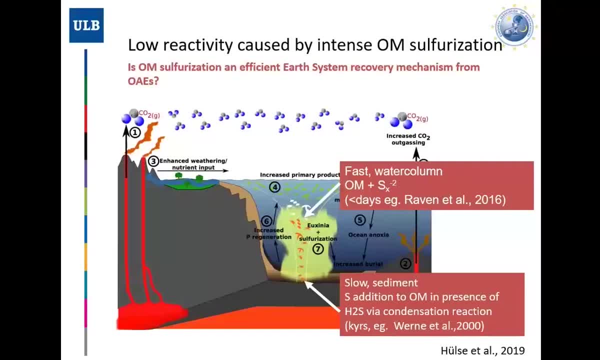 that 네 organic matter in the water column before it reaches sediment. how important is it doing that so that it has a big contribution, Like when you explain that in the Gill там also the air draft wherever you see ones around 고 organic metal sulfurization is really rapid and efficient. maybe that's an efficient earth system. 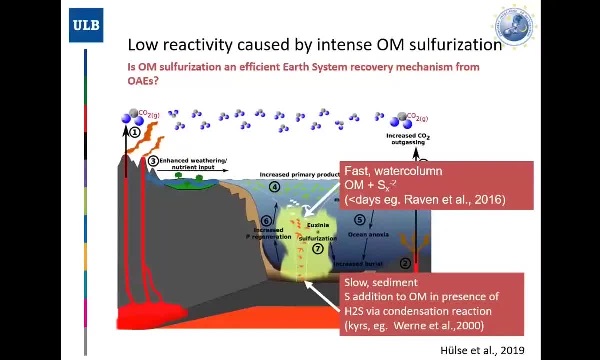 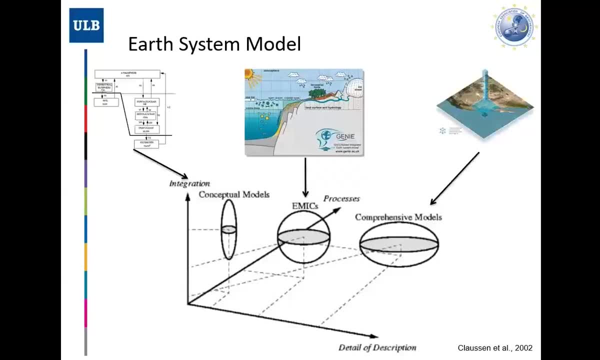 recovery mechanism. Maybe that's kind of kicking off the recovery from the OAE conditions of the earth system. So how do we test that? Now there, we have to go away from our sediment models and we now have to go to an earth system model. So there are different earth system models. 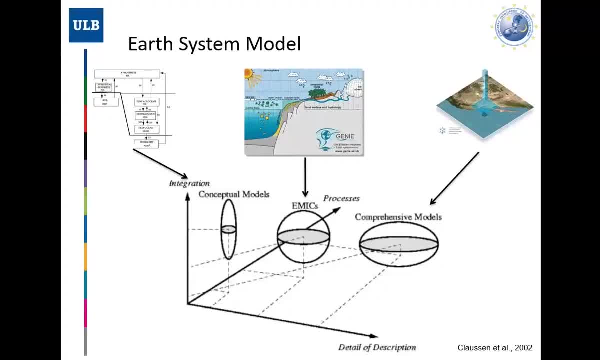 they are like different complexities. You have the typical conceptual box models, like burner model, for instance, and then you have a comprehensive models that are like, for instance, models that predict our current weather. Now, this is interesting, but it doesn't provide us with. 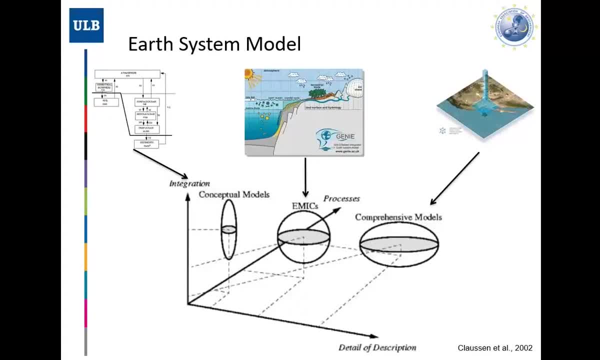 spatial resolution to investigate spatial patterns, So you could use a box model, but it's still lacking a little bit of information on the world, especially for the mutations. We do have a lot of information. we have the paleo-rejection geography. we have all the reconstructions. we have good information about where the plate 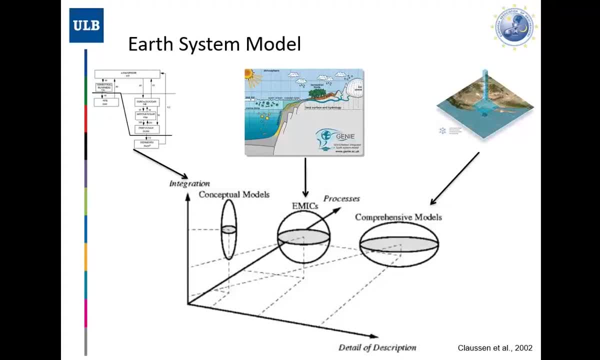 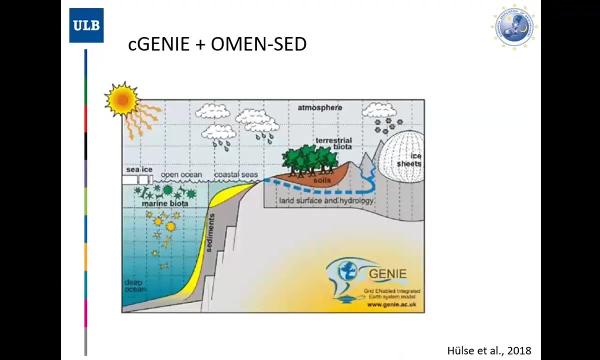 shales were found and so on, So this is often used for deeper time scales. This is something we actually use in the Banner and Zoid. These models are too computationally expensive to run for higher climates, So what we use is the TGNE Earth System model. So it resolves. 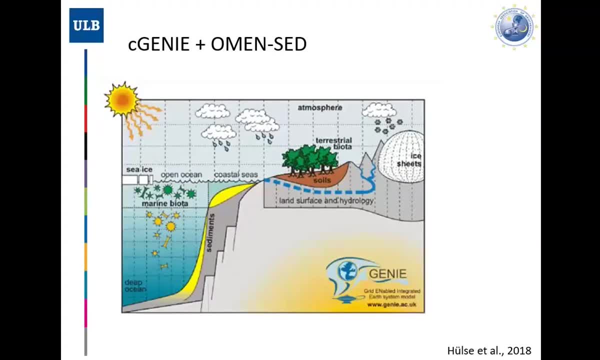 total biochemical cycles based on the atmosphere. It has a circulation scheme that catches the first quarter general circulation features. It also has a land model which we then use for these kind of simulations- simplified ice sheet And we've developed an efficient sediment model that we can couple to this model on a global scale to do these simulations. 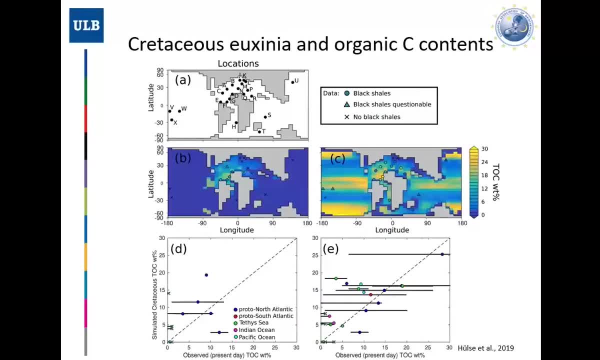 So, and with these coupled models, we then look at the results and then we look at the results of the simulations, and then we look at the results of the simulations. So we then take the sample and we then we look into the cretaceous And here you have like simulations. 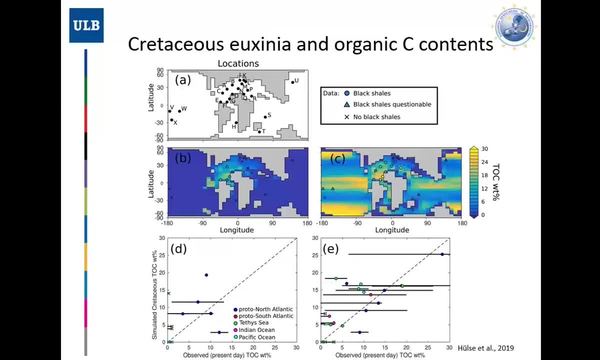 So this is pre-cretaceous conditions, This is P-O-E conditions, and here you see the organic carbon distribution over the Cretaceous world in the sediment- surface sediment- And that's over-lined by the occurrence of plate shales. So circles are, we know that they. 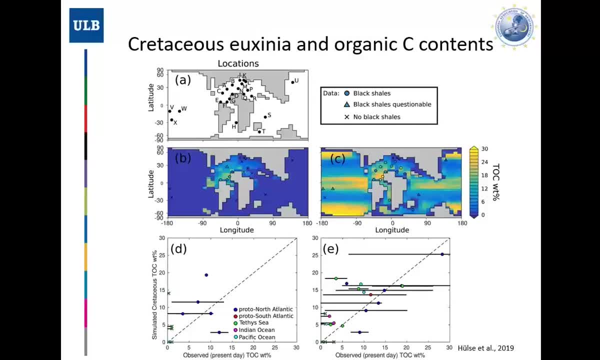 are plate shales, Thrivals are plate shales, Maybe or maybe not, And crosses, no plate shales found And we get this distribution actually quite right with the model. So this pre and this peak distribution, especially in the Atlantic. 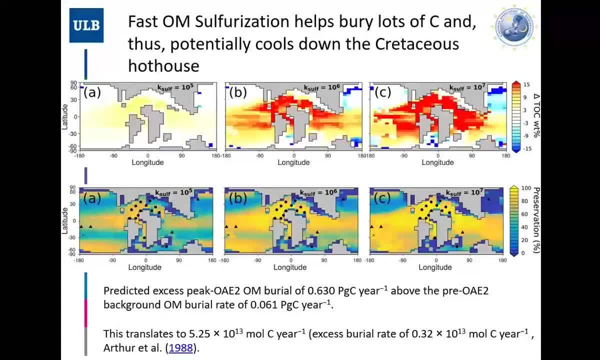 And then we lacked this organic material, sulfurite. So here you have sulfurization rates. So this is a rather low rate And then if you have higher rates, you see here is the difference in organic carbon content of the surface sediment to the normal run. 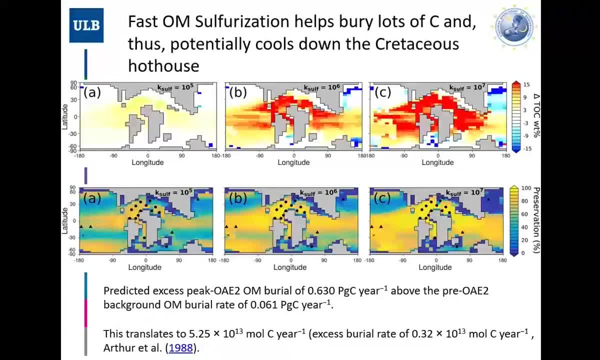 And you can see, like quite the higher the sulfurization, the higher the enrichment in organic carbon. So which means that you have, especially in these eucenic areas, a very efficient organic carbon And this fits really well With the observation. 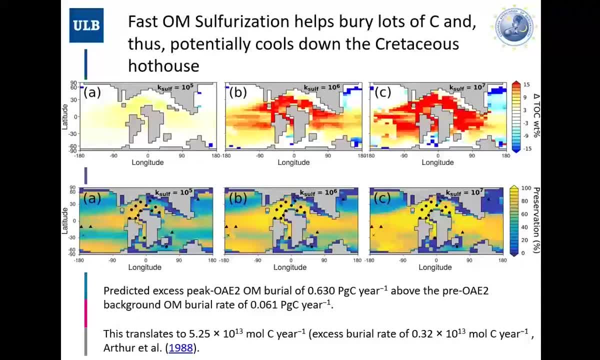 So obviously this is over predicted, So this is a very rapid one. They would burn massive amounts of carbon, But if you look at this medium range here- the rays that were also observed in carrier information- you get a reasonable transition, And so it's. it is possible to reconstruct this and see that more organic carbon gets buried. 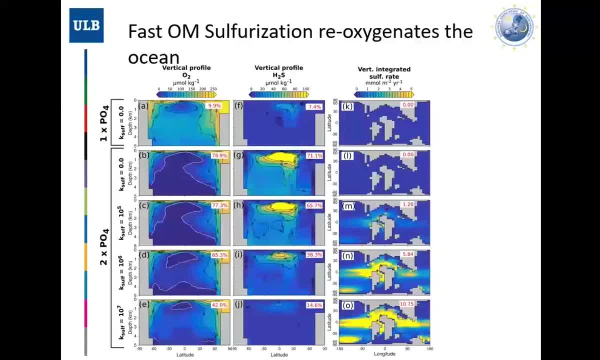 But it also has an impact on the random state of these. So here we see oxygen profiles, H2S and vertical sulfurization rates. So this is just a transect through the global ocean And here you have the global map. So this is just a global ocean and then distributed in depth. 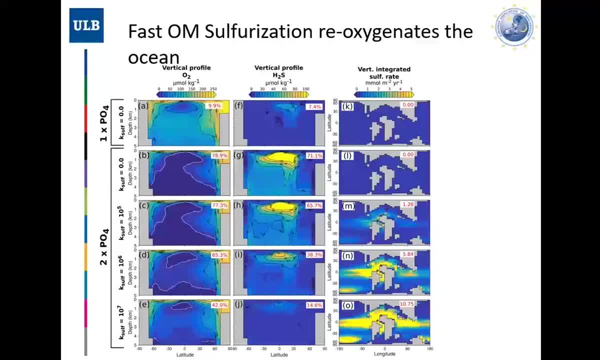 So it's one deep cut or two cuts through the global ocean Latitude and depth. So we are looking into the ocean And what we see. So this is pre conditions- no sulfurization. And then we have here OEE to peak conditions with sulfurization. 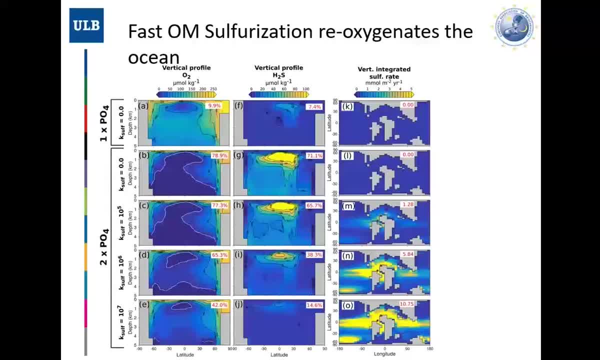 And what we see if there's no sulfurization, we have a pretty eucenic ocean, pretty epoxic ocean. There's large eucenia, Obviously no sulfurization. And then if we have sulfurization, if we switch that on, we can see how the eucenia slowly. 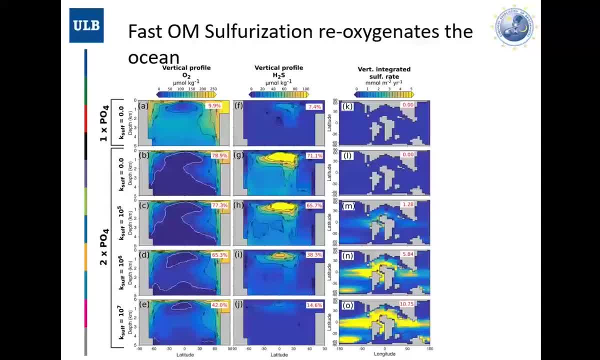 Disappears, The anoxia slowly is reduced, The eucenia disappears And you have this sulfurization. So what we see is that sulfurization is not only very efficient in burying organic material, It also helps the ecosystem in recovering from these extreme redox perturbations. 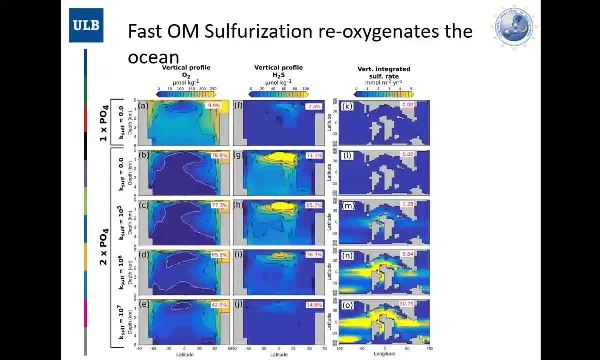 So from these anoxia and eucenia, And that will get the ecosystem back to normal mode of operation. So we bury this excess CO2.. In the sedimentary rapid, The ocean recovers from these anoxia and starts to regrade. 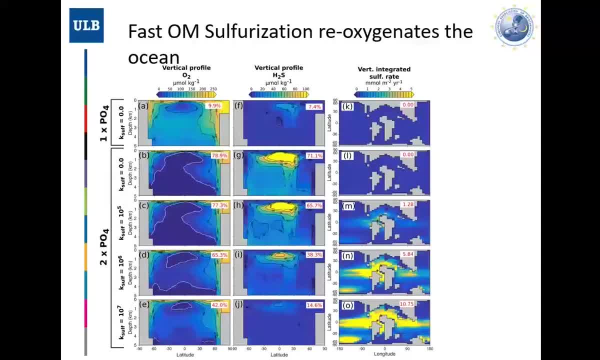 So this can really work, The first kickoff of this recovery. I think the system is complex enough. There's not only one mechanism that tried something. You see that here You obviously need high primary productivity. You need this combination of preservation To get the patterns right. 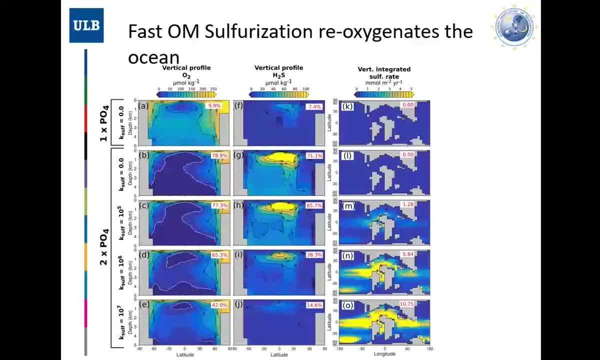 It's the same as a recovery. There are probably multiple processes at scale. They are also like mineral protection mechanisms. There is a phosphate, Phosphorus cycling that works in these anoxic sediments that can have certain feedback processes. So it's a lot of processes operating at scale. 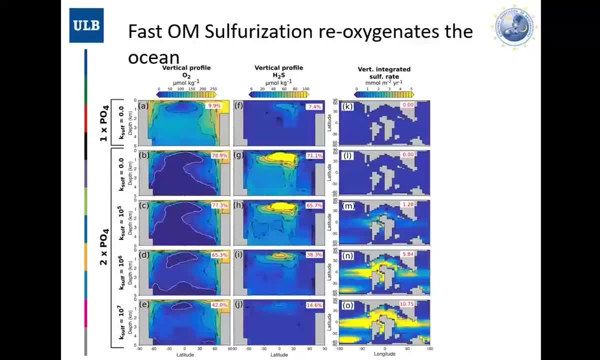 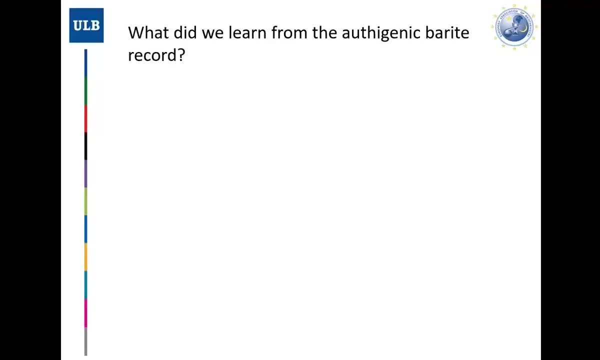 But organic matter sulfurization can play a role in helping in this recovery. So So what did we learn from these autogenic barites that really make our life normally so difficult because they really spoil our highly on productivity proxy wreck? So we've seen that even after 100 million years. 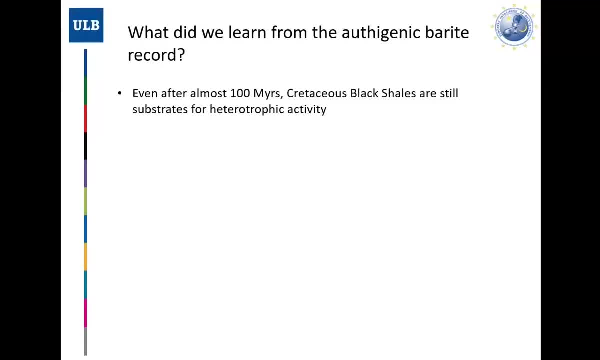 Cretaceous flexures are still substrate for heterotrophic activity in the deep biosphere And again, we still find this absolutely amazing. The organic matter is not very reactive, which is to be expected And this is important- Most probably never really was. 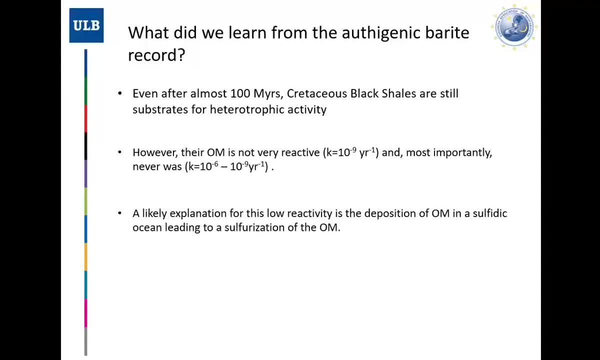 So always less reactive than what we are depositing nowadays in the modern day ocean, And likely explanation for this low reactivity is that this organic material, especially in the equatorial Atlantic, was deposited in the sulfidic ocean, leading to the sulfurization of this organic material. 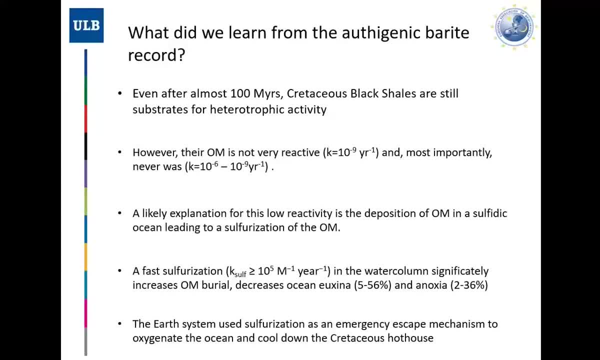 And then you see that a fast sulfurization in the water column is possible And can significantly increase the organic carbon burial decrease, urging anoxia and new senior. And it's possible that the earth system used to authorization assets Kick out the mechanism to oxygenate the ocean and cool down the contagious